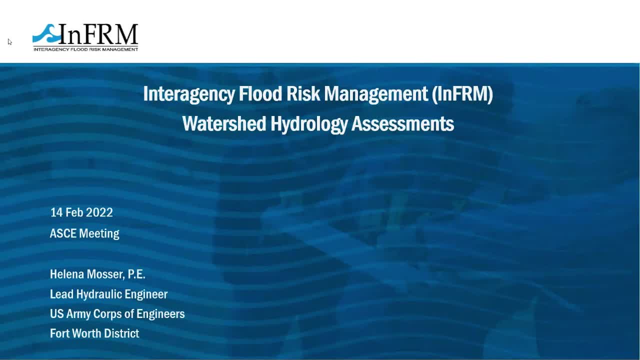 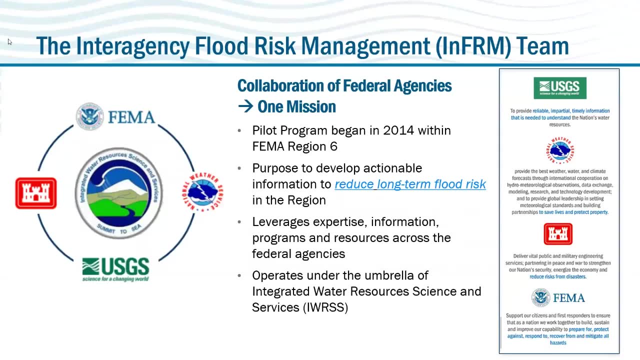 how much water can we expect to run off from the watershed, and especially for these 100-year type events? So first just a little bit about the INFORM team. INFORM stands for Interagency Flood Risk Management and it's basically a collaboration among federal agencies. It includes the Corps. 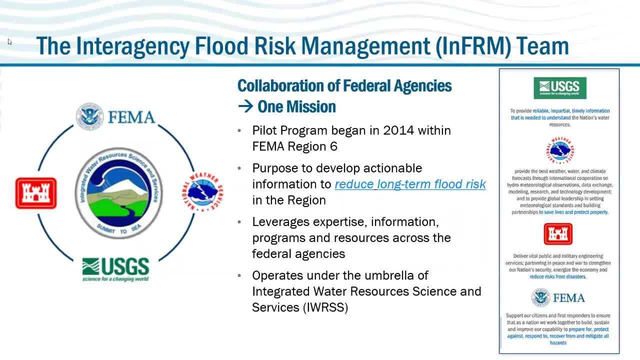 of Engineers, FEMA, the National Weather Service and the USGS- so the major agencies that are involved in water resources. We began a pilot program in 2014, where we basically are trying to leverage each other's experience, information and resources to try and reduce long-term flood risk in the region. 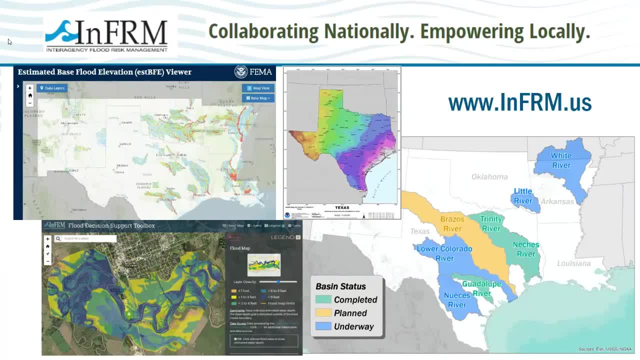 So these are some of the efforts that we've been involved in. Jerry touched on a few of these, but this is the INFORM website, wwwinformus. You can go on there and you'll find out more information about the INFORM program. So if you're interested in learning more about the INFORM program, 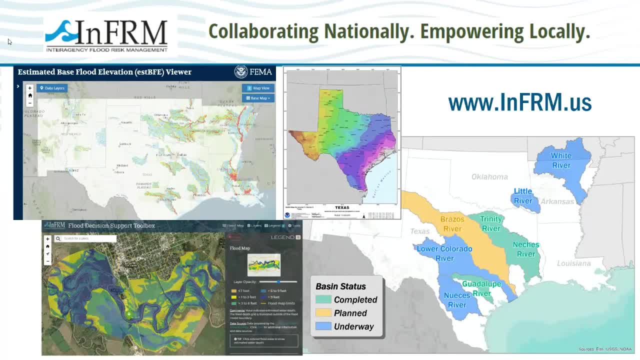 you can go on there and you'll find out more information about each of these efforts, including the Flood Decision Support Toolbox, the Estimated Flood Elevation Viewer, and then the Watershed Assessment is in the lower right there, which we'll be talking about today. 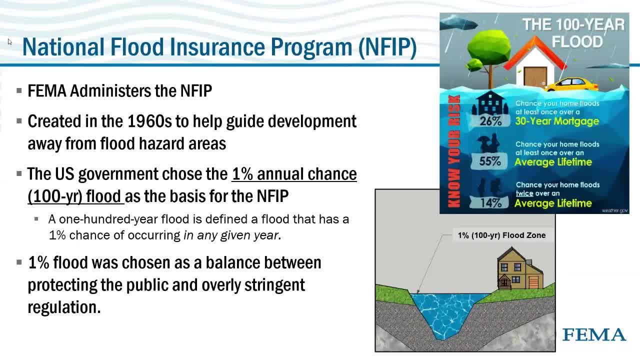 So first some background. We are doing this to support the National Flood Insurance Program for these studies, which is administered by FEMA, And so originally this program was created in the 1960s to help guide the development away from flood hazard areas. 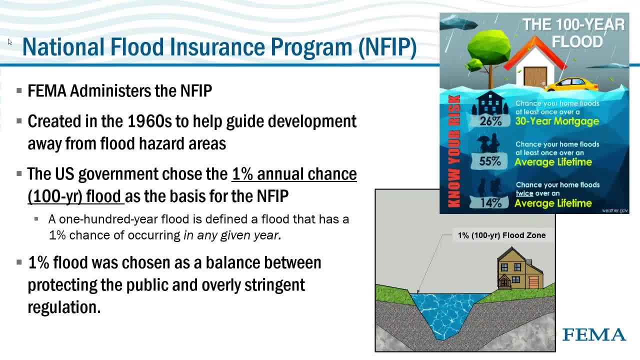 And the US government at that time chose the 1% annual chance, otherwise known as the 100-year flood, as the basis for the NFIP, And so the 100-year flow is basically chosen as a balance between- we don't want to be overly- 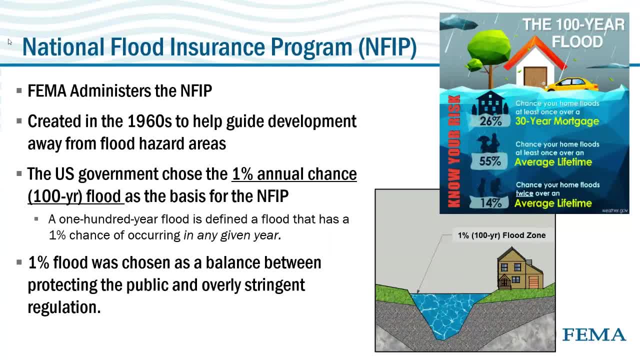 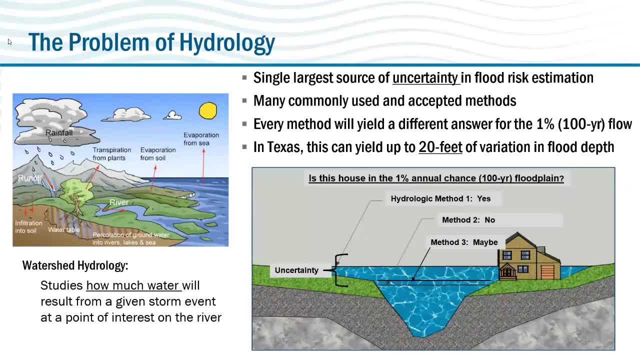 stringent in our regulation but we want to protect the public And so it's somewhat of a compromise at the standard. But the problem with hydrology is that it is really the single largest source of uncertainty in our flood risk information. You know, we have a little bit of uncertainty in our hydraulic models. We may not know exactly how much roughness there is. 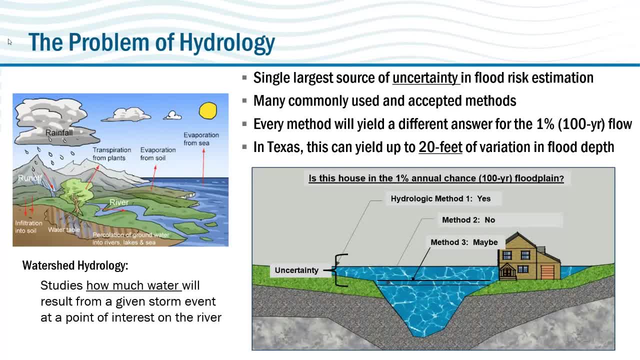 in the channel or a floodplain, but there's a lot of uncertainty in hydrology. There's also many commonly used and accepted methods, including the 100-year flow, And every method you try will give you a different answer, And in Texas we've seen that this variation between methods can yield up to 20 feet in the 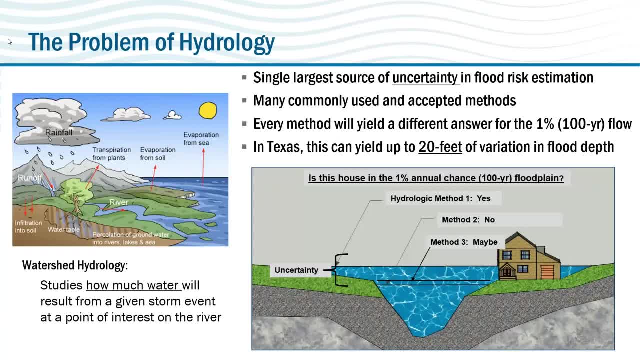 depth of a 100-year floodplain, And that's specifically in the hill country where you have a lot of variation in depth anyway. But even in this area we've seen answers seven or eight feet different in the DFW area, based on what method you're using to calculate the 100-year flow. 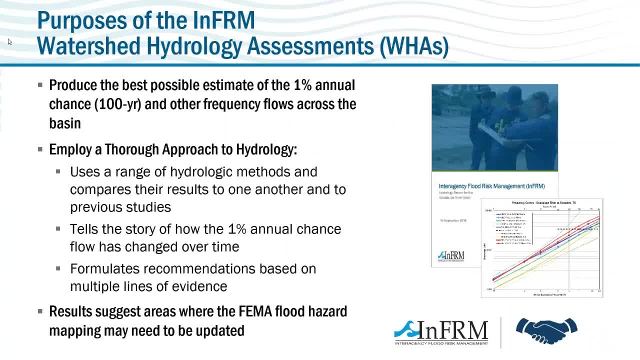 Okay, So the purposes of the watershed assessments that we've been working on are really to try and produce the best possible estimate of the 100-year or 1% annual chance and other frequency flows across the basin. So we tried to employ a thorough approach to hydrology, And what I mean by that is we use a range. 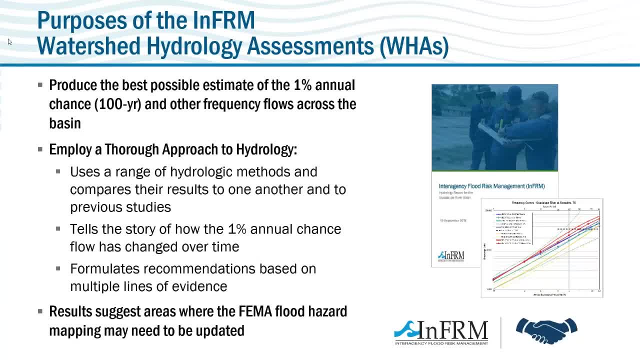 of several different hydrologic methods and then compare their results to one another as well as to previously published studies in the basin, And this helps us tell the story of how that 100-year flow has changed over time, And it also helps us formulate final recommendations based on not just one answer but on multiple lines of evidence. 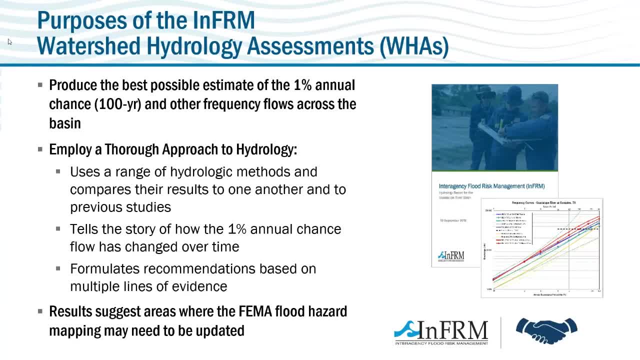 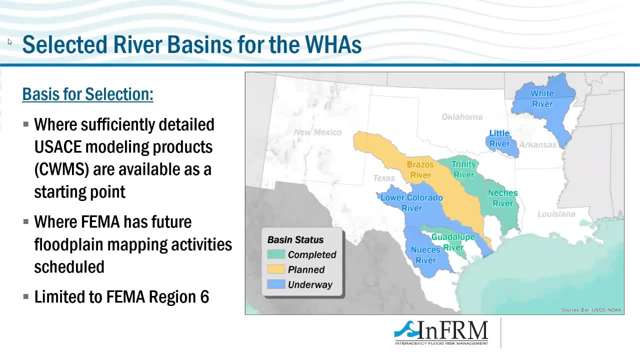 So these results that we do from these studies are used by FEMA and others to suggest areas of here's, areas where we may need to update the floodplain mapping. So this is showing how the basins that have been selected and working on so far. So in this map the green are already completed basins. 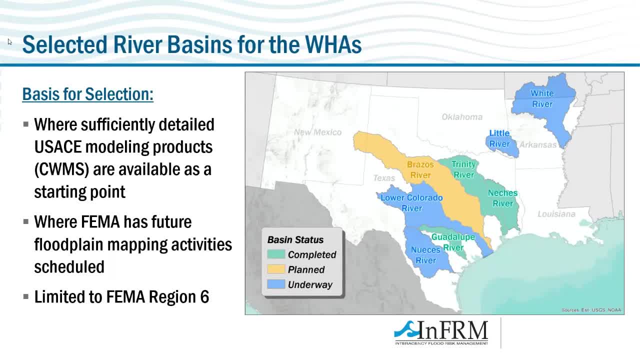 As Jerry mentioned, the Trinity River, which includes this whole area, was just published last summer And most recently, the Natchez River just came out within the last month or so. But these basins are selected based on where we already have. 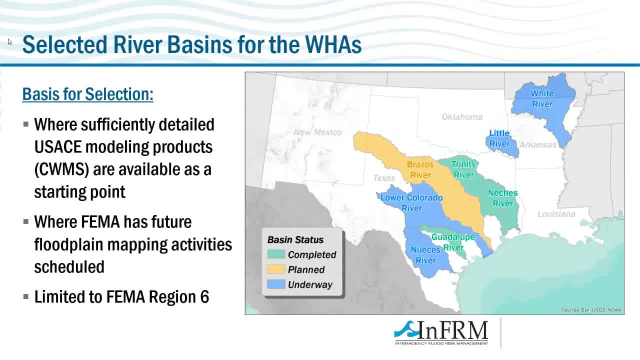 sufficiently detailed modeling products available as a starting point and then where those converge with where FEMA has future floodplain mapping activities scheduled. So right now this is a pilot program, So it's limited to FEMA Region 6, which includes Texas and the other states you see here, but it may be expanded to other areas in the country in the future. 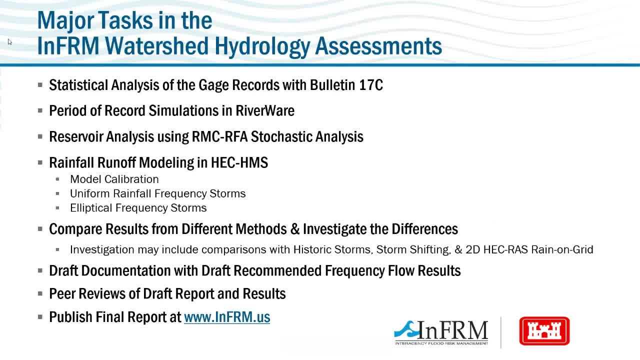 So some of the major tasks that are included in these watershed assessments are the following: The first one is the floodplain mapping. The second one is the floodplain mapping. The third one is the floodplain mapping. The fourth one is the floodplain mapping. 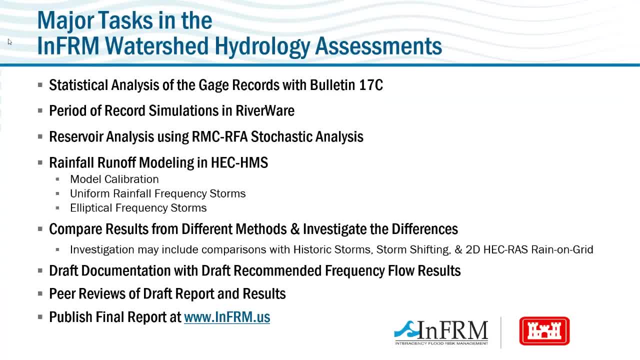 The fifth one is the floodplain mapping. The sixth one is the floodplain mapping. Include all the things you see here and we're going to go into each one of these in a little bit more depth in the remainder of this presentation, but includes 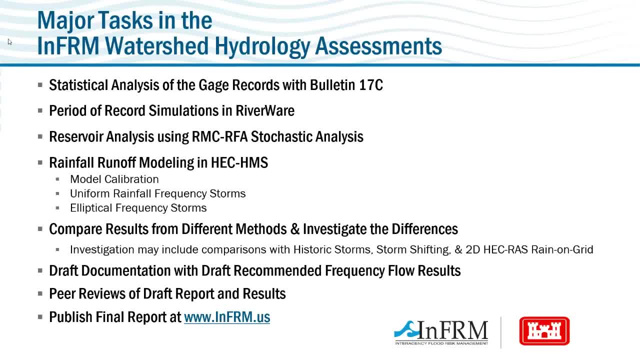 statistical analysis, period of record, simulation, reservoir analysis, rainfall runoff modeling, and then comparing those results to one another and investigating reasons for why they're different. And then we also publish a final report and we go through a peer review process. So first you'll also see the Cyclone. 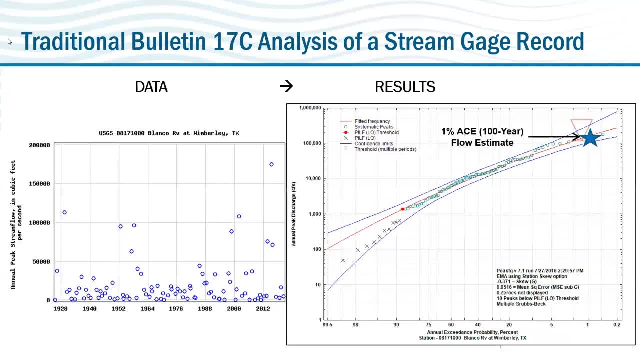 First statistical analysis of the gauge records. So I don't know if there's any hydrologists here, but somebody that's worked around this field for very long, You probably are familiar with Bulletin 17B or 17C. This is the traditional, you know, standard practice of how calculate the hundred-year flood where you have a gauge record. 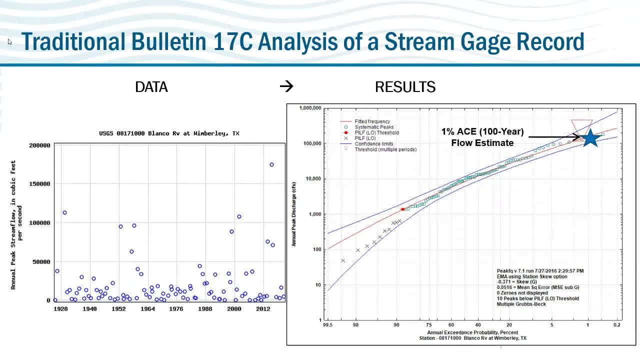 So, if you're not so familiar, what we're seeing here, the left hand graph, so that's basically a graph with the x-axis the year's record at a gauge, and then y-axis is the highest flow that has occurred in a given year at that gauge. and so you take the 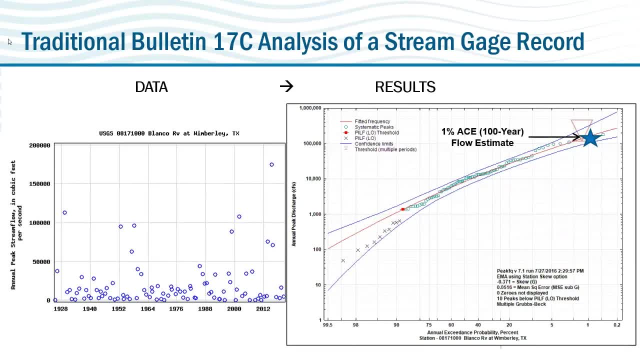 highest flow from each year and you run it through statistical procedure and that helps you come up with the frequency curve that you see on the right hand side, and that's where you have probability on the x-axis and, once again, annual peak discharge on the y-axis, and so you run this analysis pretty. 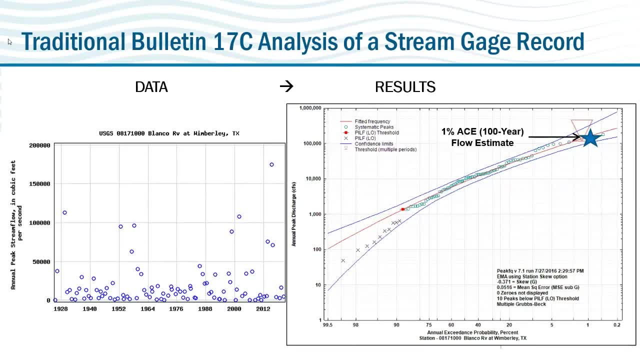 straightforward and simple. you get your estimate of 100 year and that's represented by that red curve and there is uncertainty bounds that the analysis will give you around that. but our experiences, most people don't pay much attention to those uncertainty bounds. they're like: i have the answer. that's all i need. let's go forward and move on. 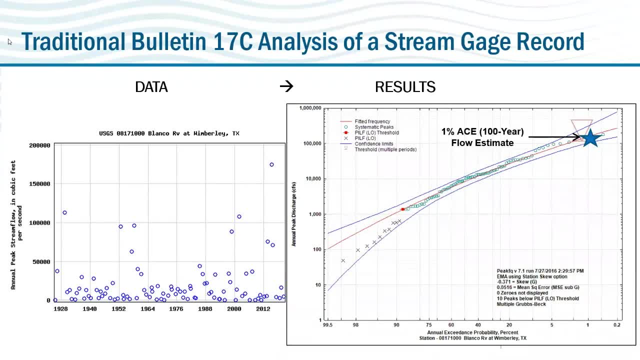 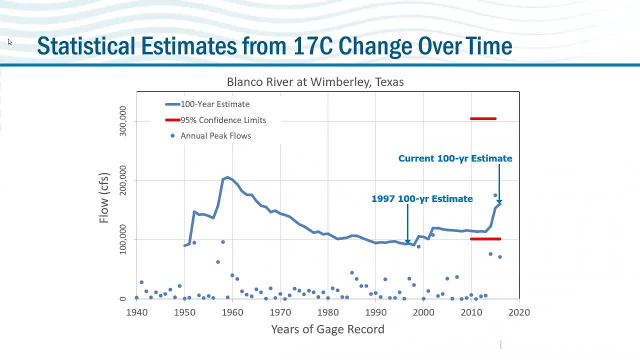 but what we did is we started taking this gauge data and we just started plotting it in a different way for these watch assessments. so this is that same data with the years of record on the gauge of gage, record on the x-axis, and that's. those points, once again, are the highest flow. 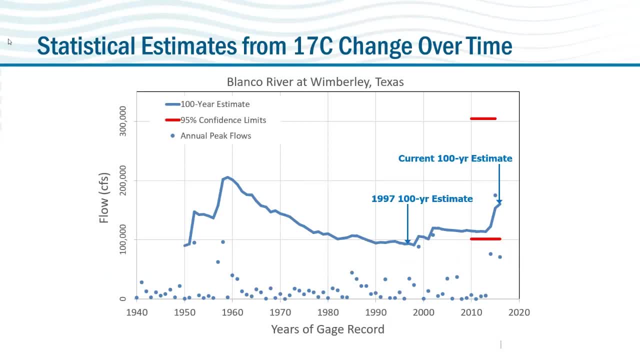 for that year and then we started calculating what is the 100-year estimate based on those statistics up to that point in time. so that is what we're going to do, and then we're going to go ahead and you just need to see how far along from this is that 100-year flow that has already started. 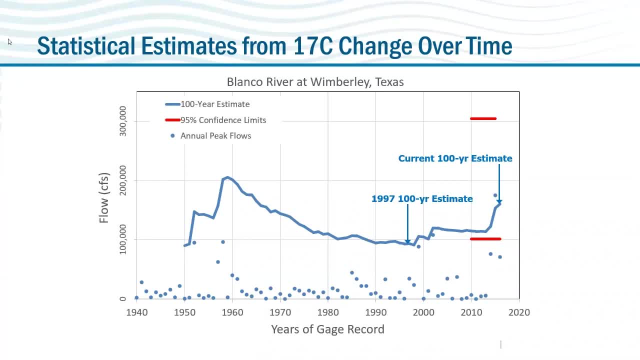 going to look and then we're going to be using this information to look at how much is going to change over the next 20 years. this is what you see in that solid blue line so you can see, based on the gage record we have, in 1960 we were calculating 100 year flow of close to 200 000, then some more. 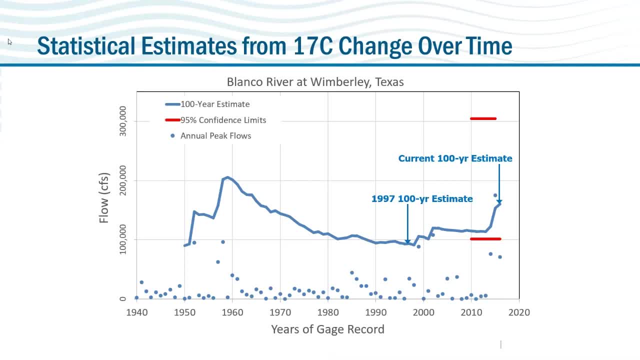 decades go by. by the time you get to about 1990, 97, that estimate has been cut in half down to 100, 000, and then we got some more floods recently and that that estimate is back up to about 150.. and so this: 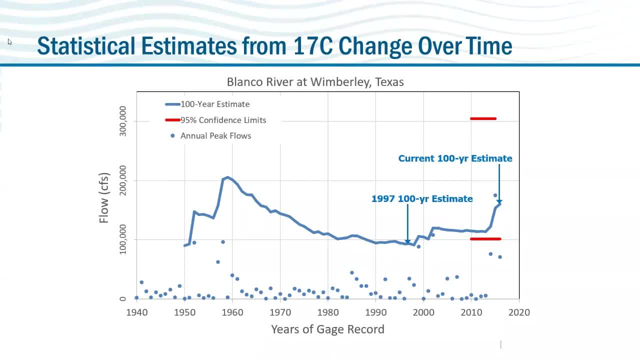 those estimates change over time, just based on your gauge record, and we're showing this example. this is the blanco river near wimberley. jerry alluded to that horrible flood that happened in wimberley in 2015.. well, the flood maps for fema at this location were actually published in 1997.. 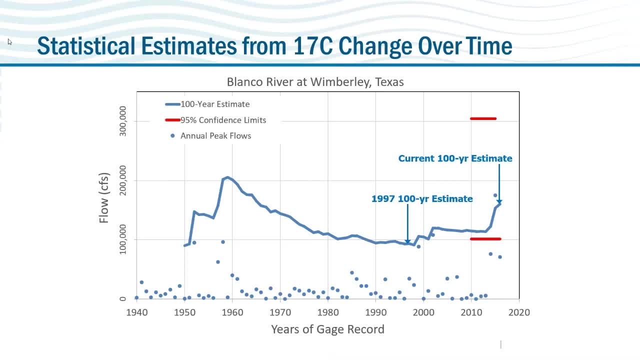 what you see on that graph is at the low point in the record. so all the flood maps that that community have were based on the lowest possible estimate at that location. so this helps us be aware, as we're looking at a gauge and analysis, are we at a relative high point in the record. 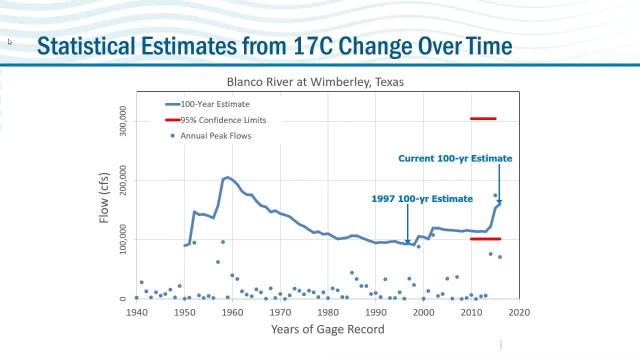 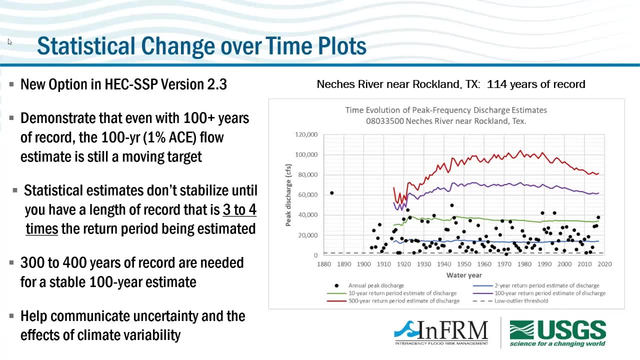 are we at a relative low point or are we somewhere in the middle? so this type of analysis- if anyone uses hec software, it's actually been added as a new option in hec ssp, which is their statistical software package, and so this helps once again when you're communicating with stakeholders or a community. 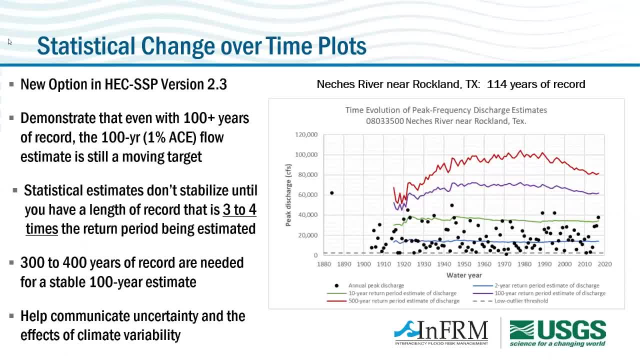 it helps communicate better than just that confidence band of what is the uncertainty in these estimates and how have they changed over time. it also demonstrates that even when you have 100 years worth of record, that 100-year flow estimate is still a moving target. this graph- 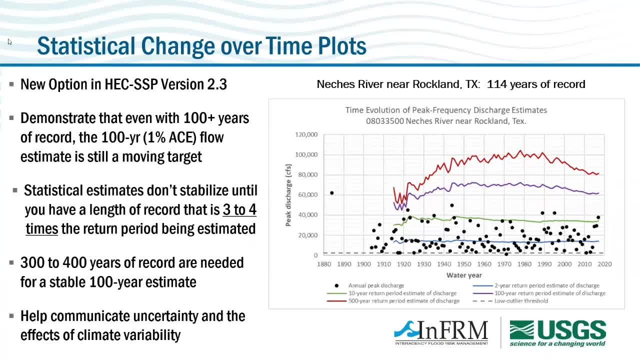 on the right is from the natchez river near rockland, texas, which has 114 years of record. that's a really long record for texas. we don't get many gauges with more than 100 years, um, but even then that that estimate, which is the purple line, is still moving and some of our statisticians 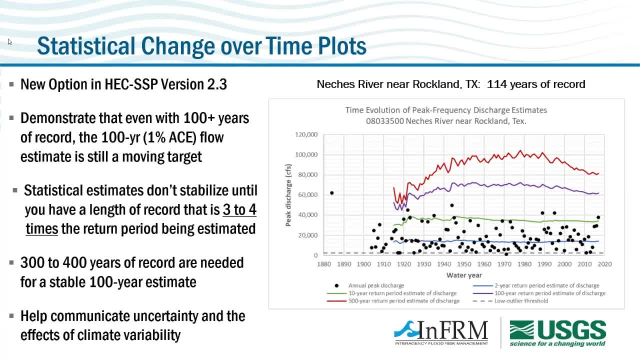 at hec, the hydrologic engineering center, have shown in their studies that statistical estimates don't stabilize for flood hydrology until you have a length of record that is three to four times the return per year. a record that is three to four times the return per year. 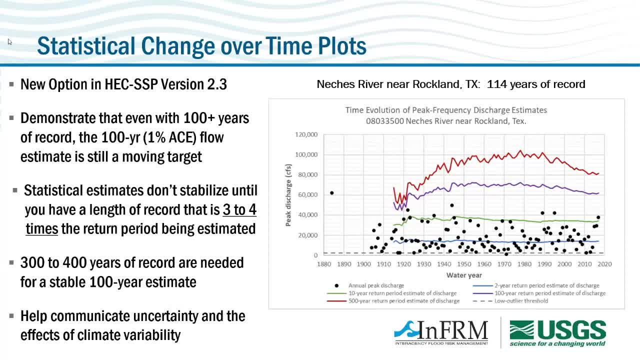 period you're trying to estimate. So that means for the 100 year you'd have to have three to 400 years for the record for it to be stable, And obviously we don't have anywhere near that in this country. But if you're trying to estimate like a 10 year flood, 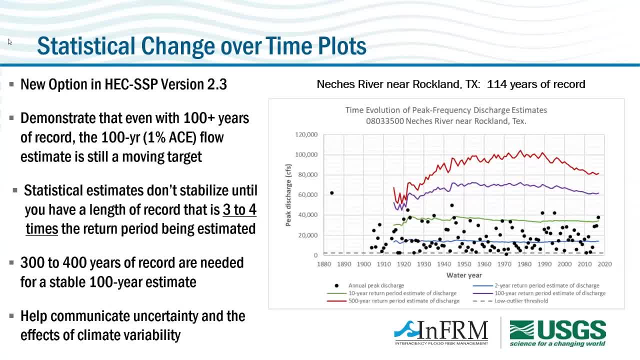 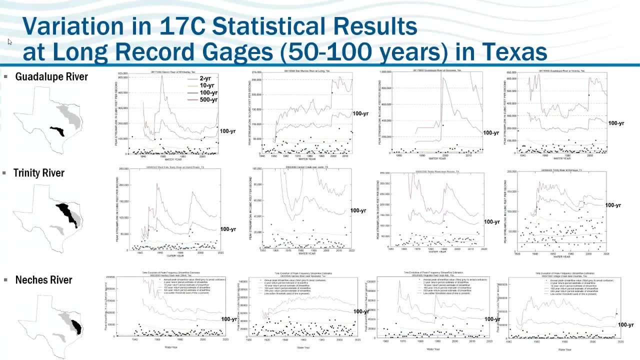 and you have 30 to 40 years worth of record, you're probably in pretty good shape And, once again, this is just another way to help communicate that uncertainty and the effects of changing climate that goes through wet cycles and dry cycles, And these are just some more examples. 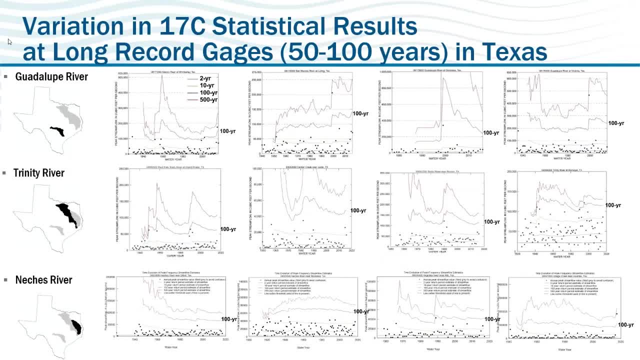 just kind of give you an idea. This isn't an isolated instance, but we've seen it all across Texas in different watersheds, different gauges. These are all gauges that have 50 to 100 years worth of record, which is considered. 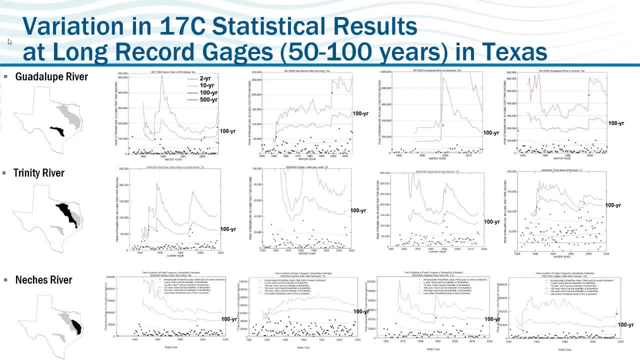 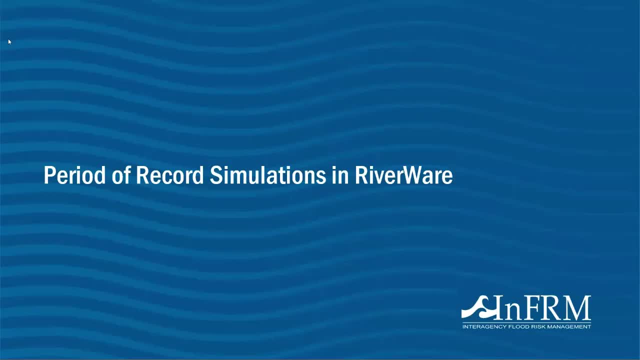 a long record gauge in Texas And those 100 and 500 year estimates are still bouncing all over the place in a lot of these locations. So next, another type of analysis we do is period of record simulations in Riverware, And this is similar to those statistical analysis. 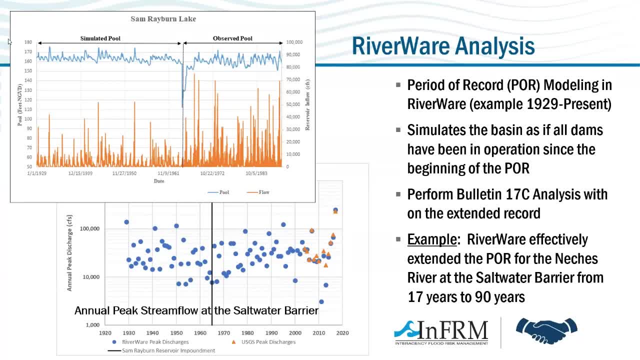 but the Riverware program is a program that allows us to simulate the reservoirs or the dams and basin as if they had been in operation in their current state for the entire period of record. So in a way it's a way to extend those records back in time. 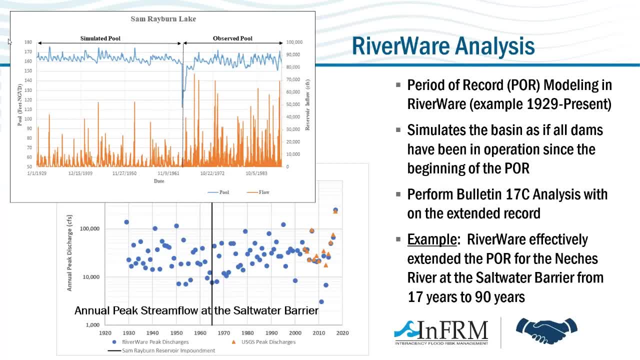 And so what you see here on the top, this is a graph, This is an example from Sam Rayburn Lake, which is the Corps of Engineers Dam in East Texas, And so we have the observed pool record, which is about from 1960, something to the present. 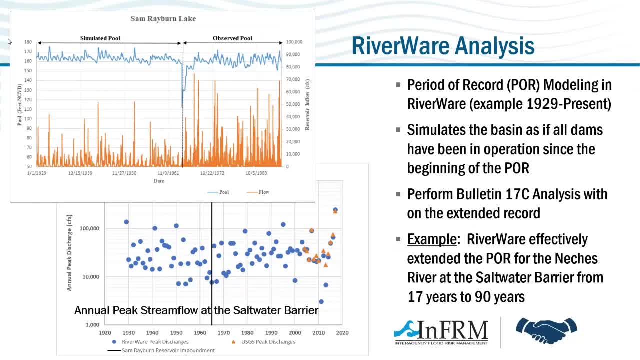 And then we have a simulated pool back to the late 1920s, And so that allows us to extend the record and understand over that last 90 years or so how would the dam have behaved? What would the pool elevations have been? 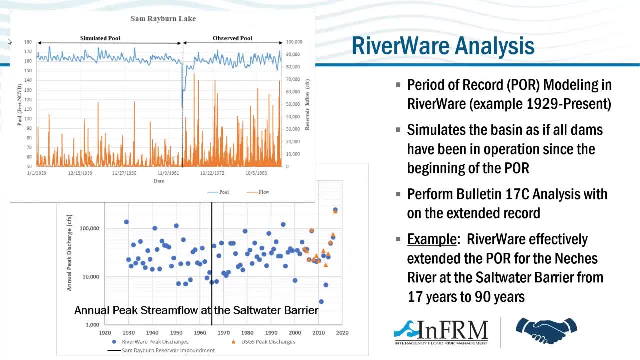 What would the outflows have been And the inflows to that dam, And so we use this analysis. One example is on the bottom there from the Natchez River, which is at the saltwater barrier down near Beaumont Texas. 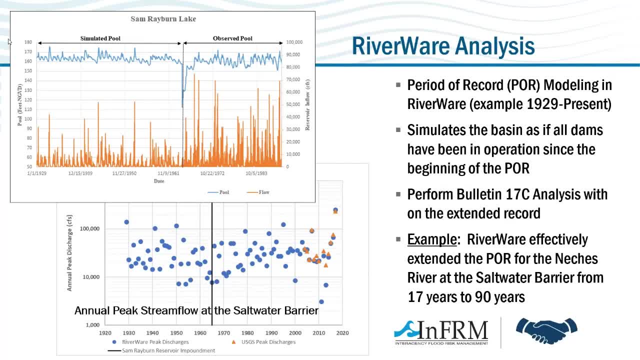 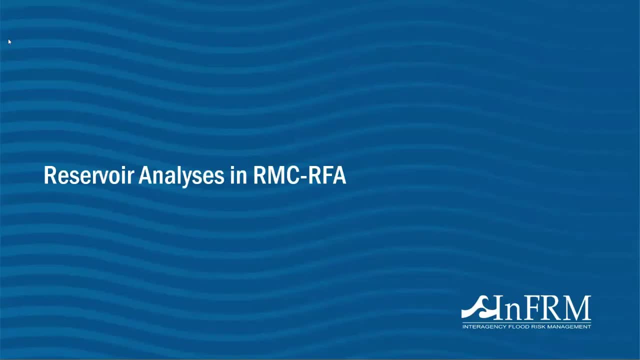 And the Riverware analysis allowed us to effectively extend the period of record for that location from just 17 years of observed data to 90 years using the old Riverware analysis. Another analysis that we use is doing a more detailed analysis of some of the reservoirs in these large basins. 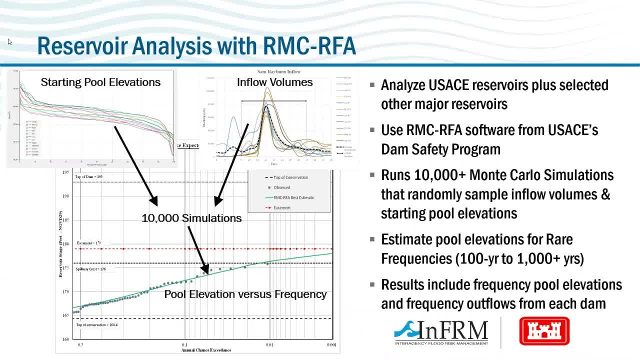 that we're studying, And so for this type of analysis, we use a program from the Corps of Engineers Risk Management Center called RMC-RFA, And basically it allows us to do a little bit of fantastic Monte Carlo simulations based on the data we have from the reservoirs. 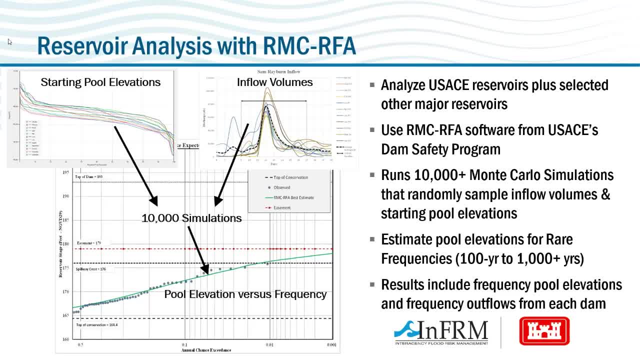 So you can see on the graph here we'll have a range of starting pool elevations that we've observed at the reservoir. We'll have a range of different inflow events, inflow volumes and hydrographs And then we can run it through this program. 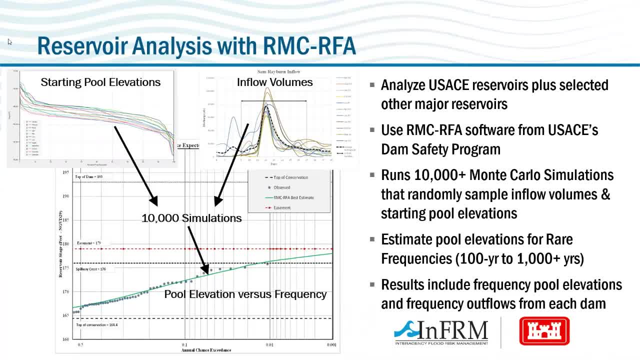 and perform 10,000 simulations, So extending the data rather than just what. we've observed all the different possibilities of what different combinations of inflows and starting elevations and what effect that would have on the dam. So this gives us a better estimate. 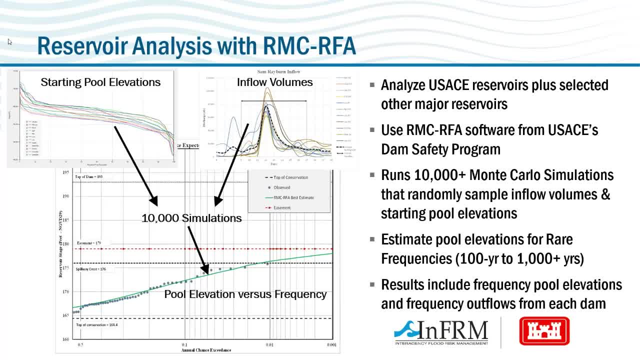 of those rare frequencies of the reservoirs, especially for things like major dams like Lake Louisville. you'll pool some of the major core dams here in the Metroplex. As far as dam safety is concerned, the dam safety community is really concerned with those very rare events. 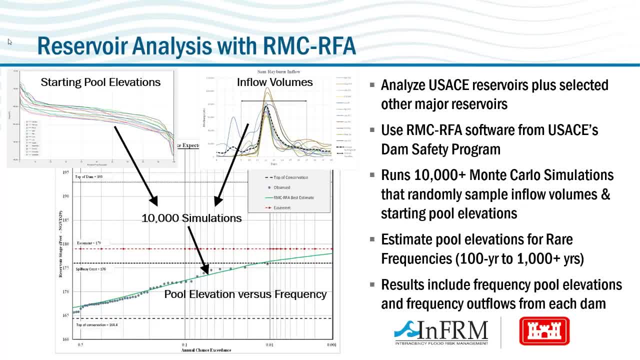 even up to the probable maximum flood. So they use this in the dam safety side of the house also to get a better estimate of those rare frequencies of the reservoirs. So this gives us a better estimate of those rare frequencies to get a better understanding of the frequency. 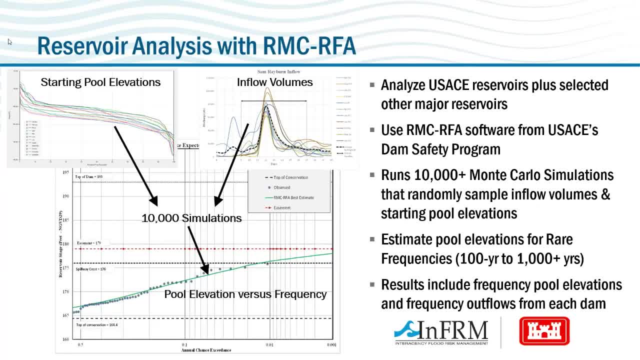 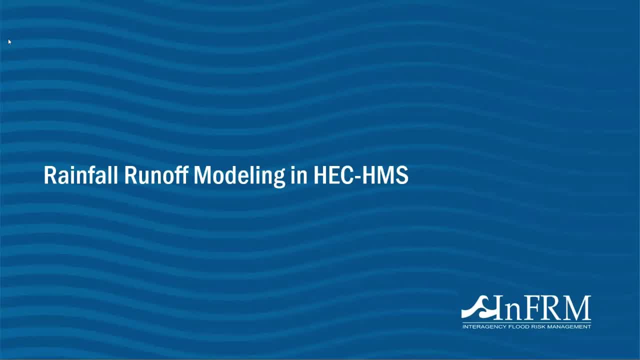 of those very, very large events, like the 40 inches of rain that Jerry had some examples of in the last talk. And then, finally, the last major piece of analysis that we do is in rainfall runoff modeling, And for that we use HEC-HMS. 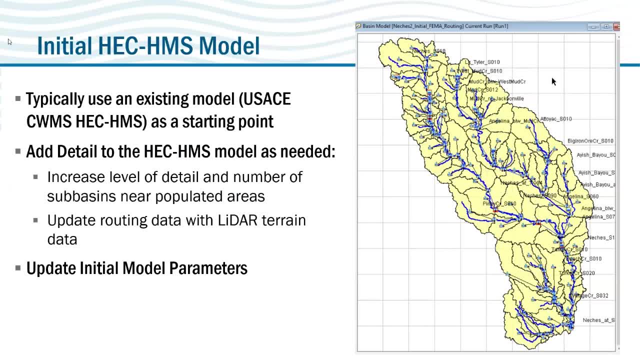 which is another free software available from the Hydrologic Engineering Center of the Corps of, and. so typically for these analyses we start with an existing model. The Corps has existing models available for a lot of these large watersheds in which we have reservoirs in operation. 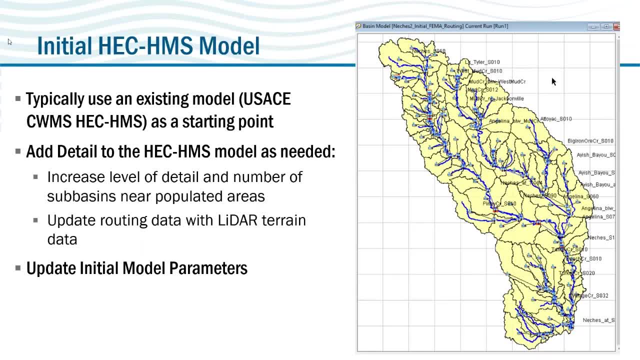 So we'll use that as a starting point and then we'll add detail as needed for these studies on the watershed hydrology assessment So we may increase the level of detail in your populated areas or update the terrain And based on new LIDAR. 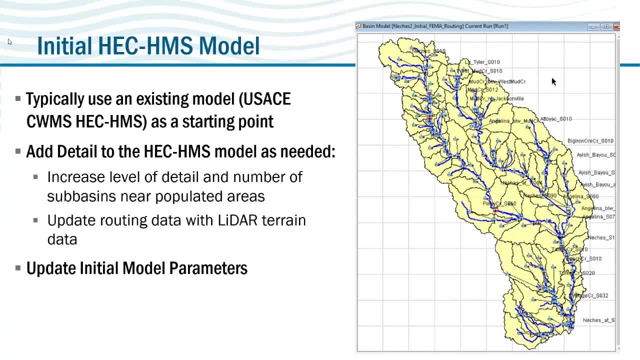 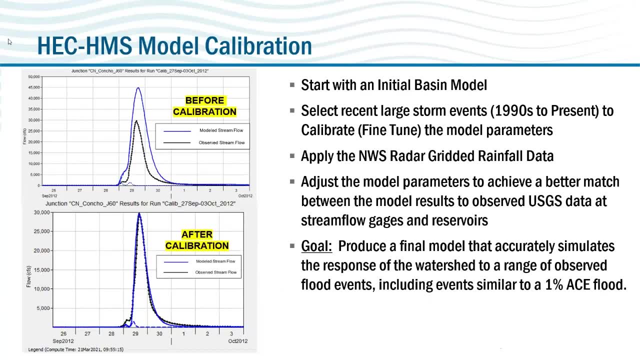 and then update the model initial parameters based on that For these studies. we also try and spend a lot of time with model calibration, And model calibration is basically where we can compare our model results to the observed results at the gauge in terms of flow for a recent storm event. 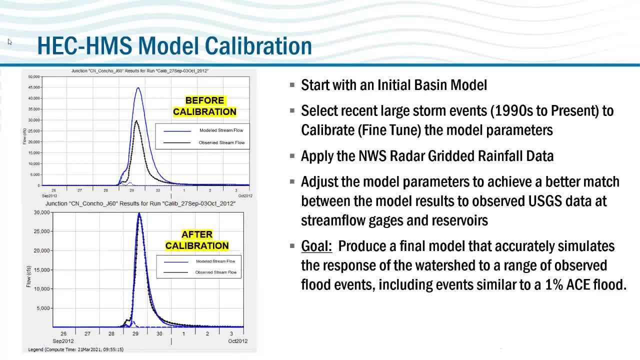 and fine tune those model parameters so that we can be sure that our model is accurately representing the response of the watershed, especially to larger flood events similar to the 100 year, which is what we're most interested in for these studies. So we go through this process. 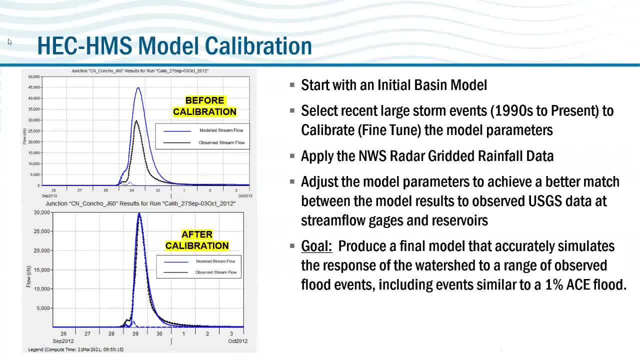 We select several recent large storm events from 1990s to present, which is time period that we have gridded radar rainfall data available from the National Weather Service, And then we'll adjust those model parameters to get better results. And that's what you see. 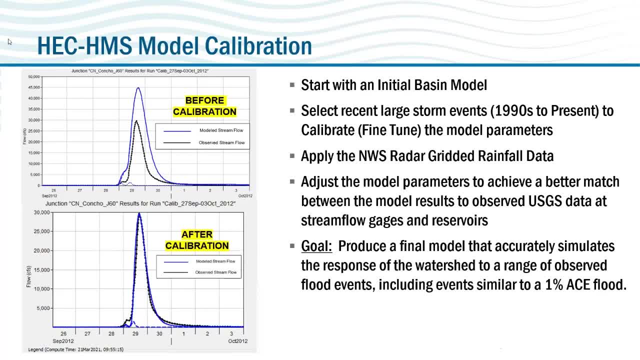 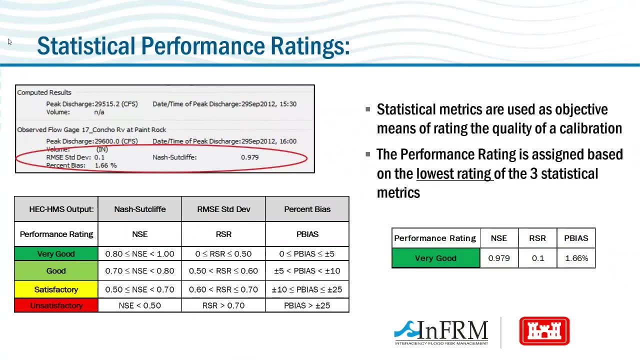 On the left there is blue is model result versus black is the observed stream flow, And we'll adjust those parameters to try and get the best match possible that we can. When we perform these calibrations, we'll also use some performance ratings just to give an objective means to quantify. 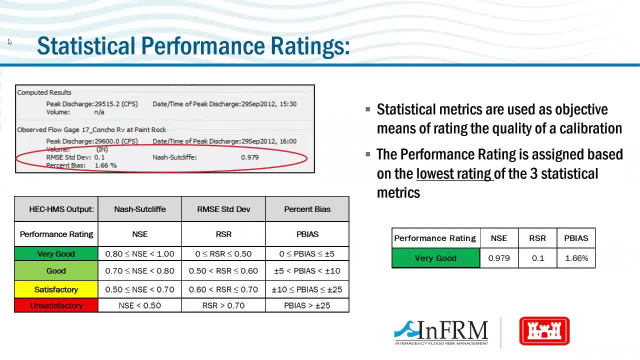 how good or bad a calibration is, And so these are some of the statistics that automatically the HMS model will spit out for you, And we'll use those to grade it from very good, good, satisfactory, unsatisfactory- on quality of the calibration. 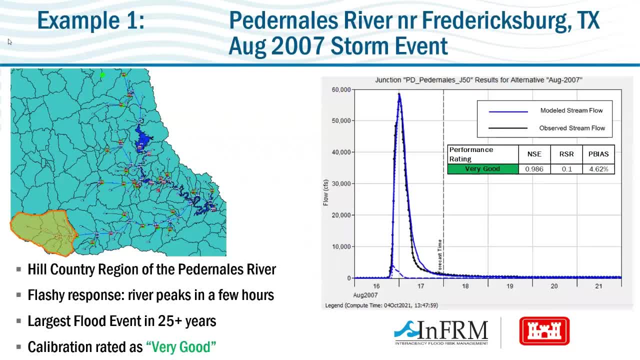 So here's just a couple examples. This is the first one, which is for the Perdonales River near Fredericksburg. This is in the hill country region, So very steep, very fast watershed response. You see the river there peaks within just a few hours. 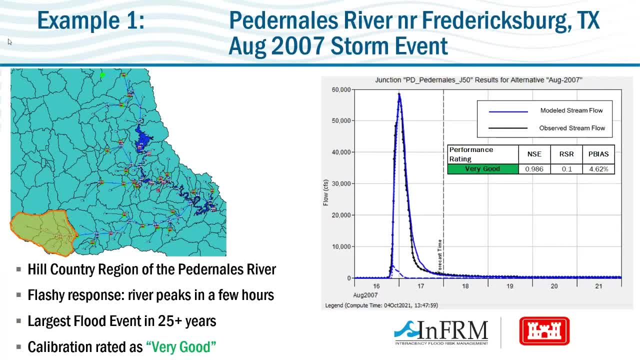 And then it comes down very quickly also, And so this was for the August 2007 storm event that occurred there, which was the largest flood event that happened at that location in at least 25 years, And so this was rated as very good. 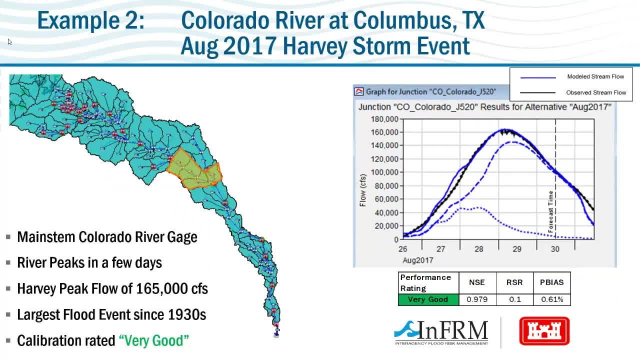 And then this is another type of flood event. This is on the Colorado River at Columbus, which is downstream of Austin, And so this is from Hurricane Harvey actually, but you can see here the watershed response in that graph of the black is once again. 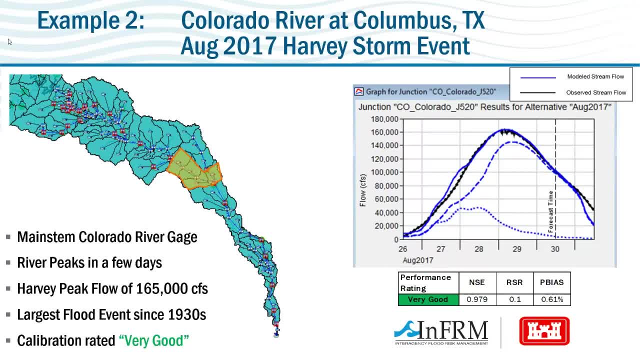 the observed streamflow and the blue is model results. Once in this example you have a very different watershed response. It's slow to rise and slow to come back down. It takes days for the river to peak at this location because you have such large area draining. 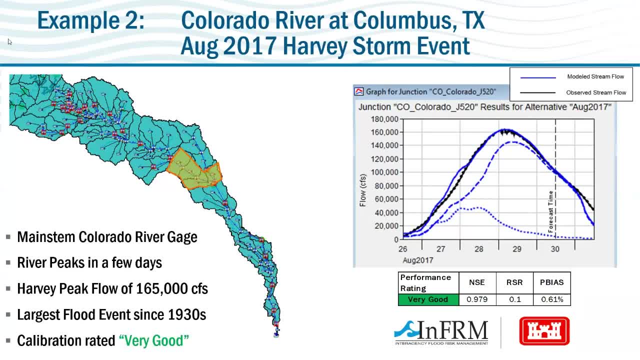 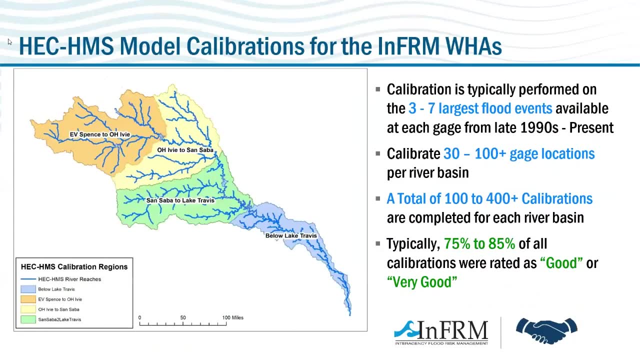 into the Colorado River And so, at this location, Hurricane Harvey was the largest flood event that had been seen there since the 1930s, which was another very wet and stormy time period for the Colorado Basin. So, all in all, for these watershed assessments, 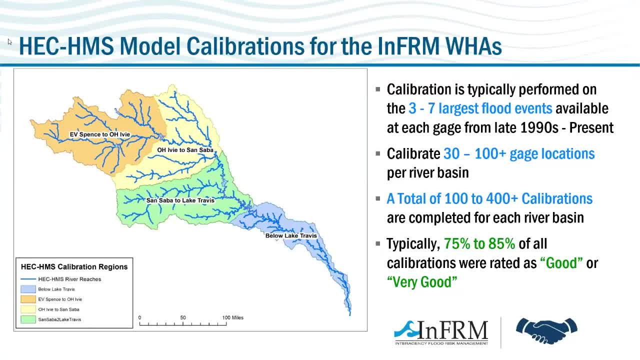 we typically perform calibration on between the three to seven largest flood events have occurred at each gauge. depending on what data, what events are available And and depending on what data, what events are available And and depending on what data, what events are available. 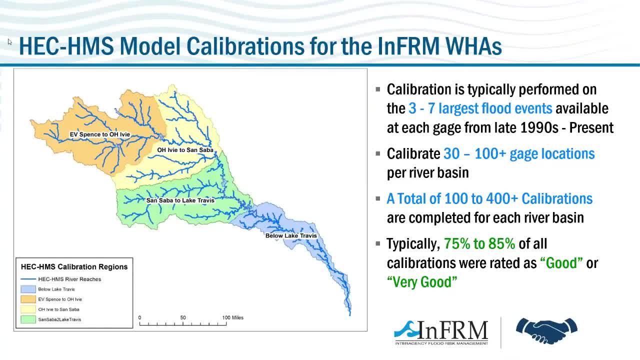 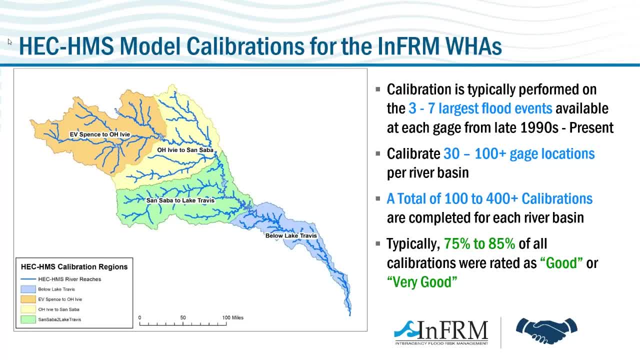 that we're studying right now and is in progress, And so we have well over a hundred gauges spread out throughout the Colorado Basin, which includes the whole Austin metropolitan area too. So, total, by the time you add it all up, we're performing anywhere from. 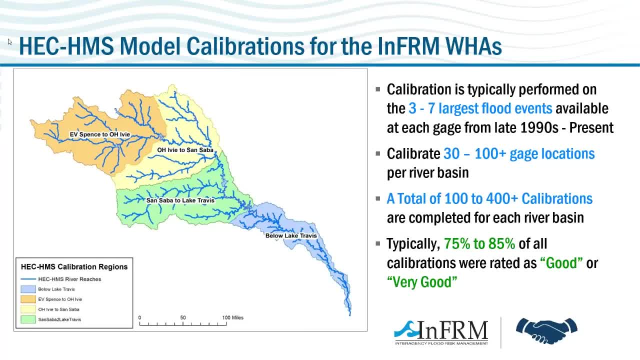 100 to 400 plus model calibrations first, you know, first adding up each storm at each location, and typically somewhere between 75 to 85 percent. the calibrations for these studies are rated as good or very good. the ones that aren't. a lot of times there's some problem with the input data. 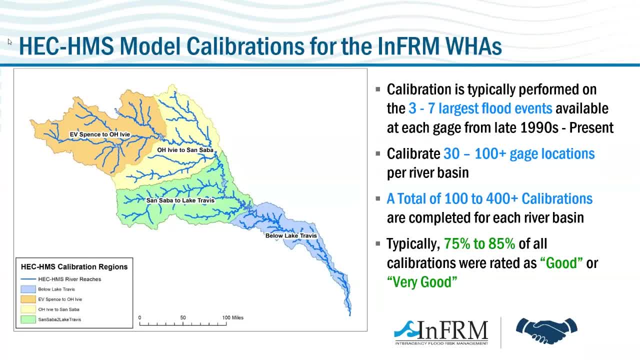 maybe the rainfall data for a certain event might have might not be totally accurate, there might be inaccuracies, or sometimes there's uncertainty in the rating curve at the gauge, and so we'll try and look at. for the ones that don't work out so good, what are, what are possible reasons for that? 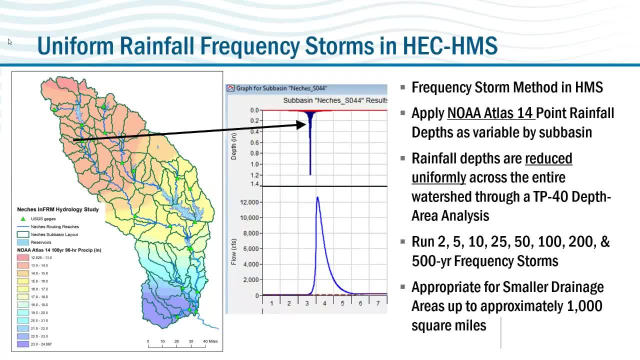 so, after completing the calibration process for these watershed models, we will then run frequency storms in the models which this is showing, that traditional method of calculating frequency storms. we apply those noaa atlas 14 point rainfall depths in the model and we'll vary it by sub basin. on the left there that map is showing a map of the. 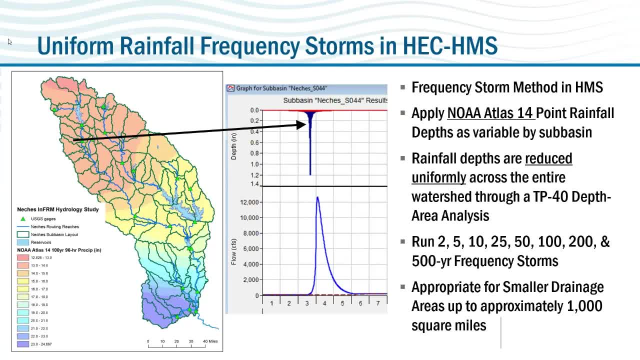 natchez river basin, which is about 10 000 square miles just in east texas, and so you can see from the north end of the basin to the south end that 100-year rainfall varies from about 12 inches at the northern end all the way down to 20 something inches at the southern end near. 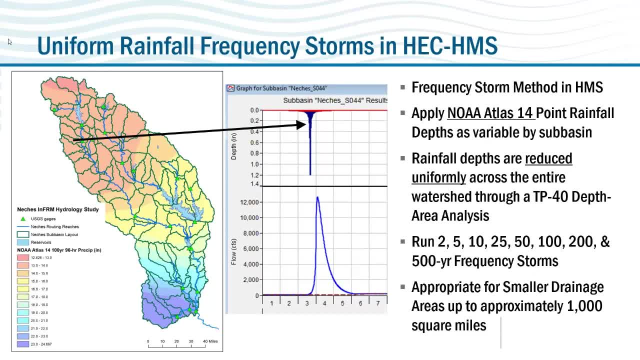 beaumont. so there's quite a bit of variation in that 100-year rainfall estimate across the basin. but the traditional method is, you know, you can put in all those different rainfall depths as variable for each sub basin, but then using what we call the uniform rainfall. 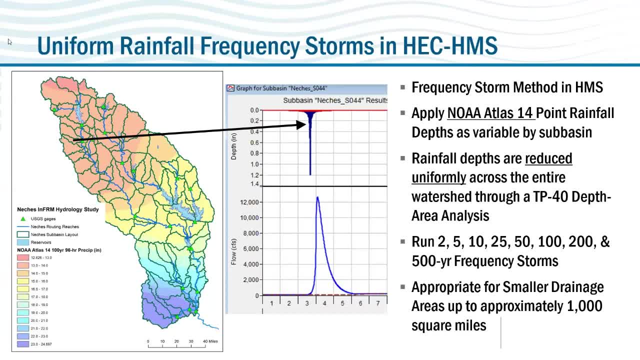 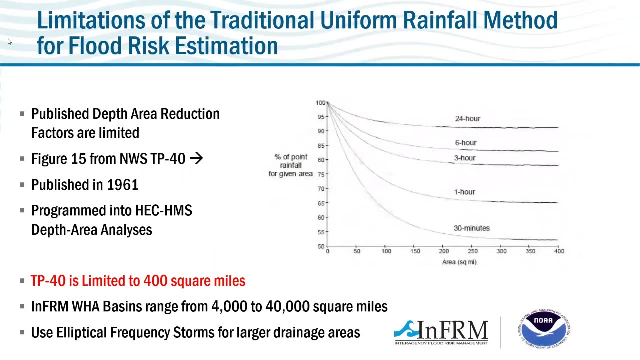 method, all those rainfall depths are reduced uniformly across the watershed based on the area you're trying to analyze. so this method is primarily most appropriate for smaller drainage areas. so by that i'll i mean up to approximately a thousand square miles. but some of the limitations of that method is that they're based on these tp40 depth. 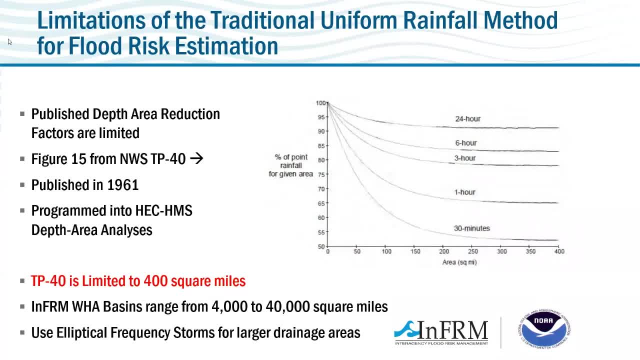 reduction factors, and so that graph on the right is figure 15 from tp40, which was published in 1961. there really aren't a lot of good, solid depth area reduction studies that have been published since then, so these curves that are from tp40 are what's already programmed into hms, if you try. 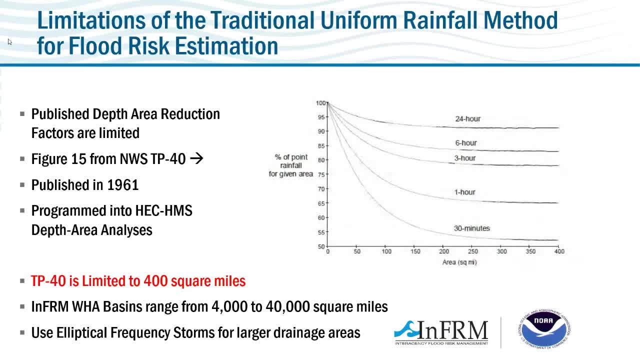 and do a depth area analysis, it will use these curves. but the problem is the tp40 only studied data out to 400 square miles, and that's just because they were limited on the amount of data that they had at that time, whereas basins that we're studying are anywhere from 4 000 to 40 000. 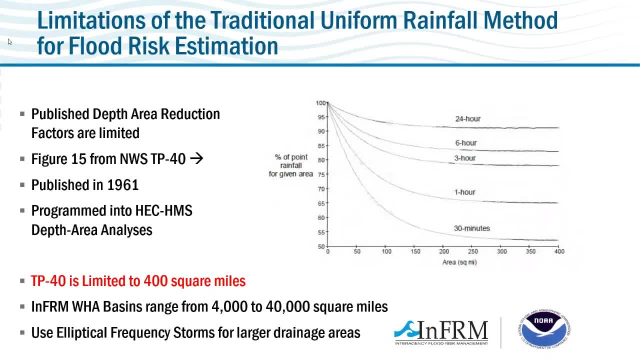 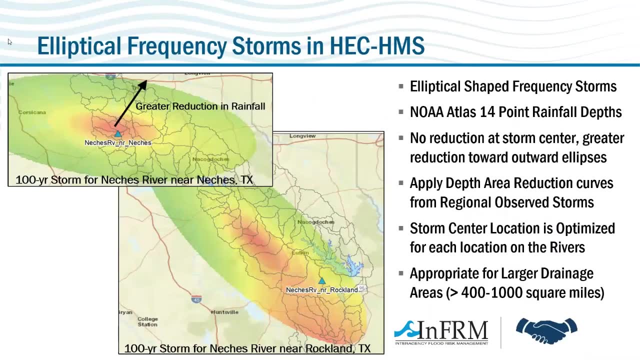 square miles. so, to account, to better account for those how the storms move and are reduced, for these very large basins and drainage areas, we started applying elliptical frequency designs to these watersheds. that's what this slide is showing a couple of examples. once again, we are still using that noaa. 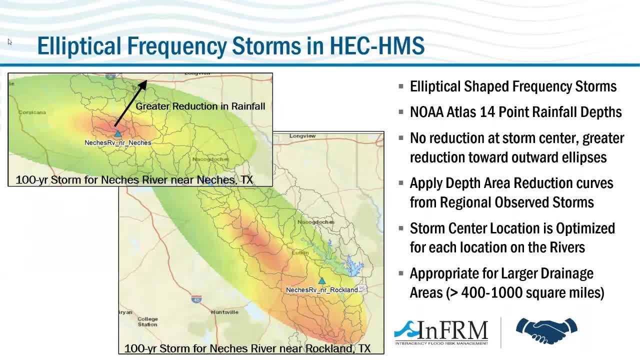 atlas 14, rainfall depth at the center of the storm and then that depth is reduced as you move outward from the storm. and the depth area reduction curves that we're using here, especially for those areas that are larger than 400 square miles, are coming from regional observed storms that we've calculated. 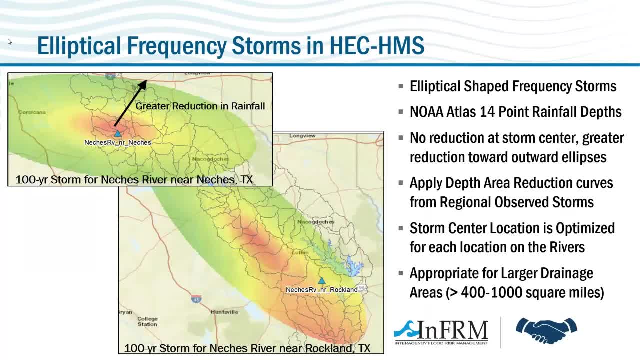 so we moved these storms around and we actually find the optimal location to put the storm above each location of interest on the watershed. so that's why you see these two different storms. these are both for the natchez watershed. one is above the 100-year storm, above natchez river, near natchez. 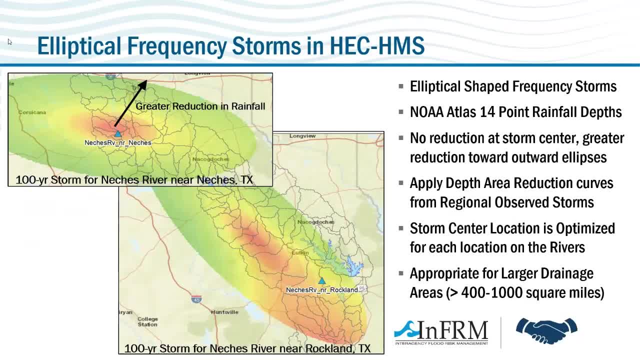 texas and then, as we move further down on the natchez river, that storm will move to an optimal location above the gauges near rockland. so these this method of applying rainfall to a rainfall runoff model and and estimating the 100-year and other frequency storms is more appropriate for the larger drainage areas. 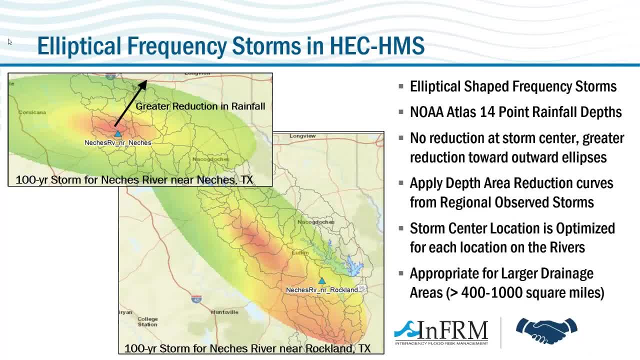 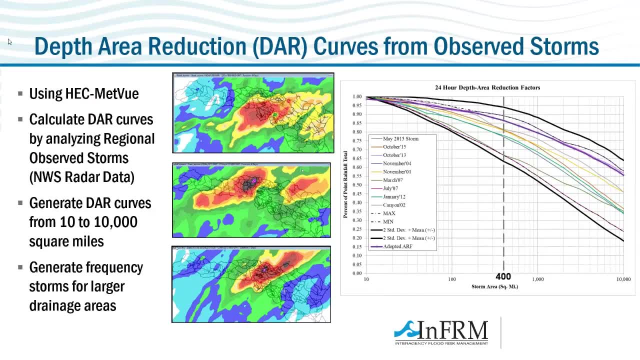 of 400 to above a thousand square miles. and then this is just showing a little bit more about how we calculate those depth area reduction curves. this is some examples of just using observed results. this is just to show how we can use this to calculate the depth and depth area reduction curves. 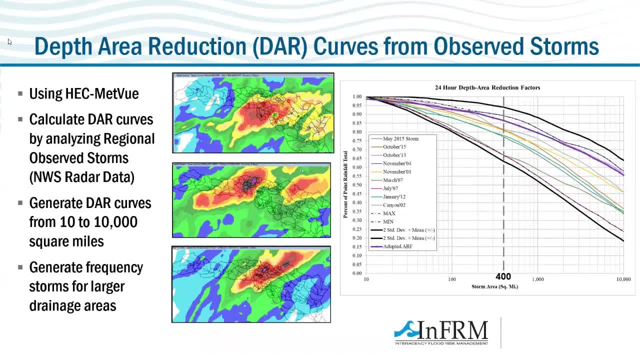 so we've done this once again in agc metview, which is a free program for processing rainfall data, and so we'll take the hourly rainfall grids from the national weather service for a storm and calculate, you know, based on the highest point rainfall for that storm, and then, as you move out, 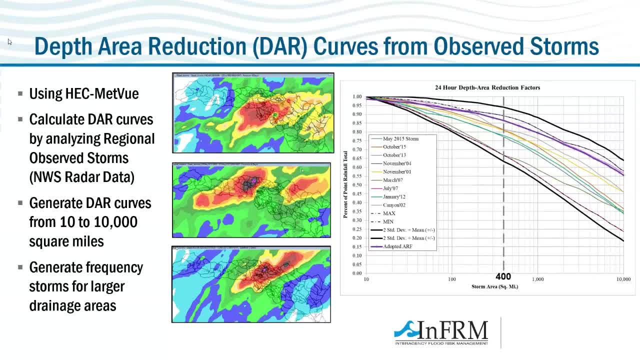 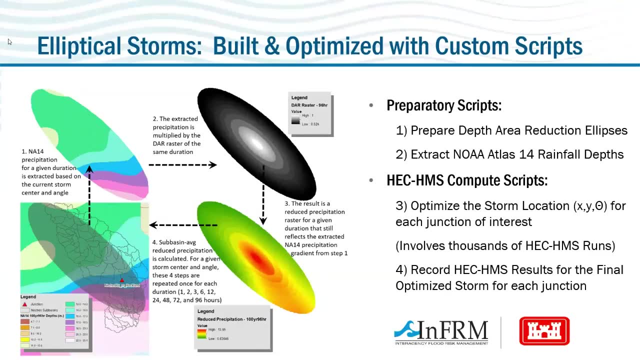 how does that depth point area reduce as you move out from the center of the storm rate? depth area reduction curves up to 10,000 square miles based on these storms, these recent storms that we've seen in the region. And then, once we do that, we 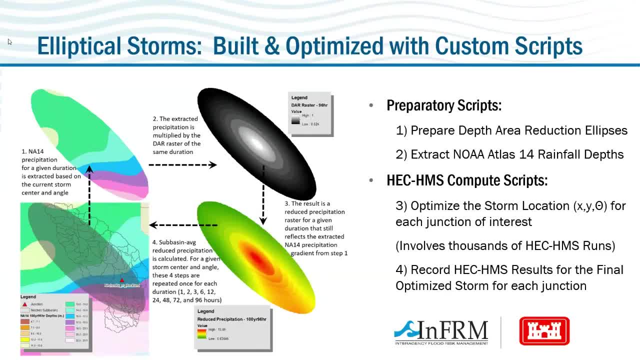 have some custom scripts that we've built to actually build the elliptical storm itself, And the diagram on the left is showing kind of the general process of taking the NOAA Atlas 14 grids and extracting the data and then applying that depth area reduction raster And then when you merge those 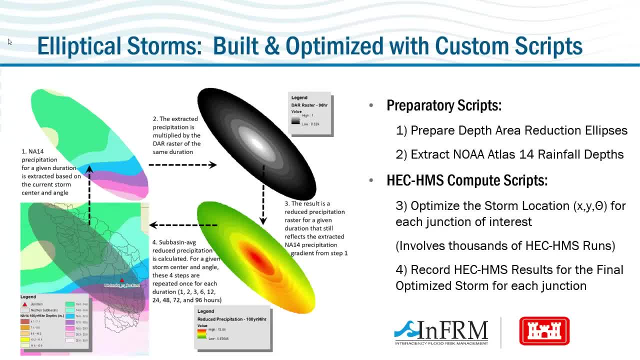 two together you get a reduced NOAA Atlas 14 rainfall for a given duration that you're interested in. We're actually working with HEC now to eventually get some of these scripts integrated into the HEC And then we're going to be working on the software itself in a future software. 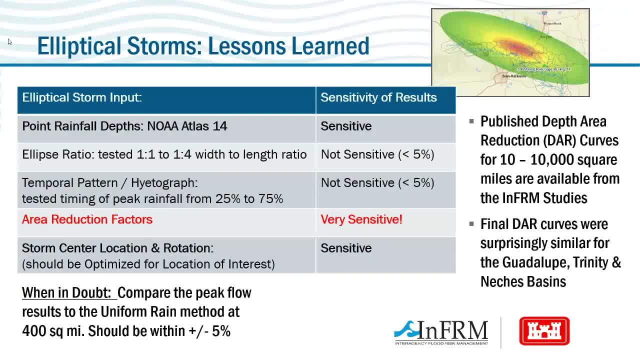 release most likely. So some of the lessons learned that we've learned from modeling and studying these elliptical type design storms: There's some factors in the elliptical storm input that it's very sensitive to and there's factors that it's not really that sensitive And so we've done a lot of testing some sensitivity. 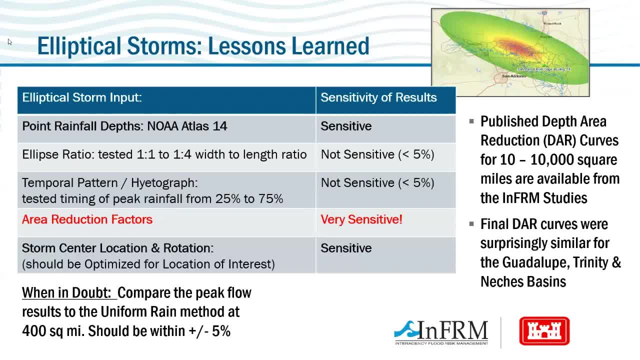 tests to see what we need to look out for The first row. obviously it's sensitive to the NOAA Atlas 14 depth, as it should be On the bottom. it's also sensitive to the location where you put the storm. 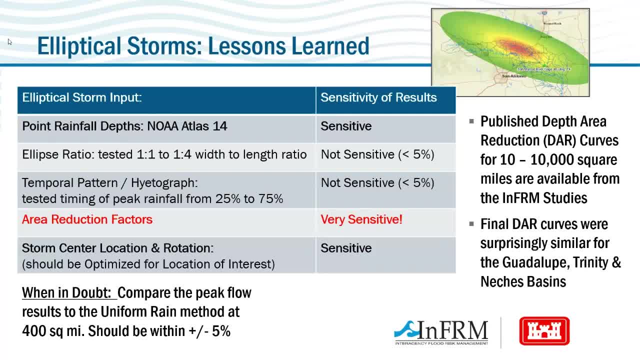 But we found that it is very sensitive to that area reduction factor, And so that's where it's important to really look at a lot of those regional storms that have happened, to make sure that the area reduction curves that you're applying are appropriate for the watershed that you're looking at. 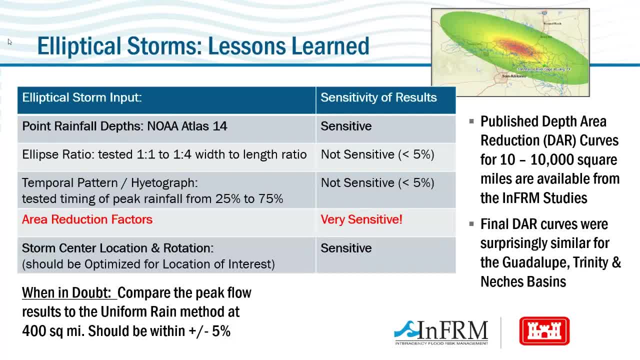 But other things, like the ellipse ratio, which is the x-axis to the y-axis of the shape of the storm, even the temporal pattern of the storm, of the rainfall over time, not very sensitive to those, Maybe plus or minus 5% in the results. 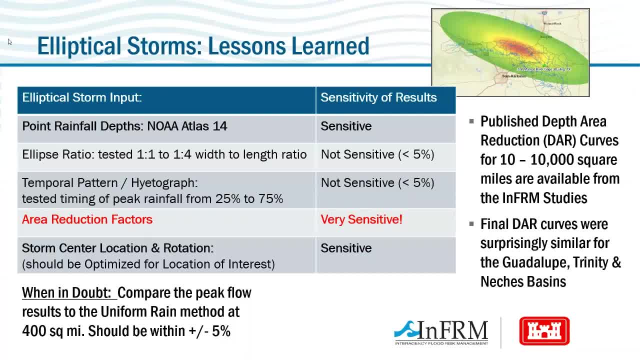 So we have some published depth area reduction curves that have come out of these InForm studies And one of the surprising things that we found is that those depth area reduction curves from different regions of Texas really didn't change very much. We have ones that we saw from the Guadalupe River down in the 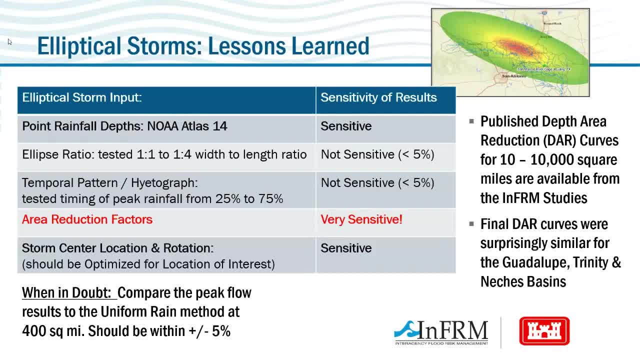 hill country from the Trinity River in this area and then the Natchez River in East Texas, And they're all surprisingly similar in how that point. rainfall is produced by area, So that's a resource that's available also if you need to apply this type of analysis. 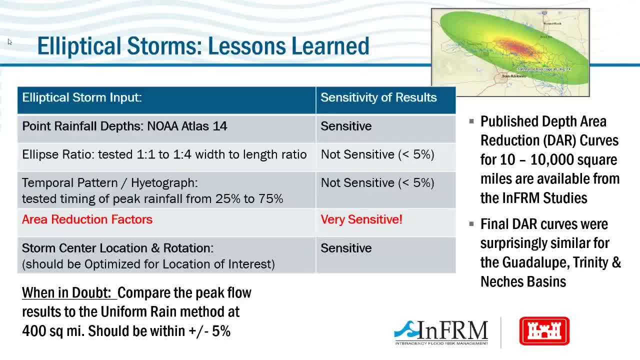 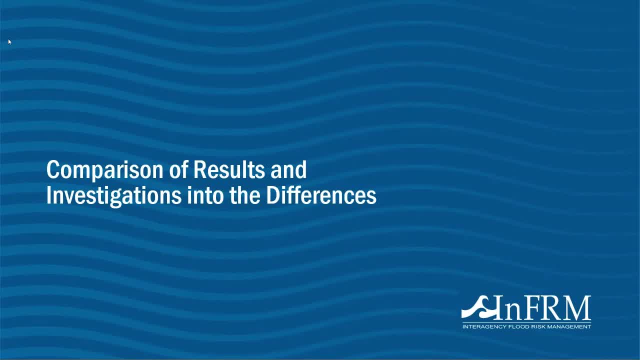 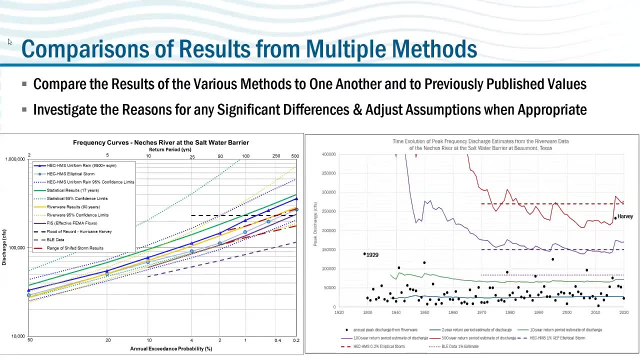 That you could. you could just use some of those already published curves, Alright. so once we finish all these basic analyses, we take results and we start plotting them in different ways, comparing them to one another. So these are just a couple of different types of plots that we'll do. The one on the left. 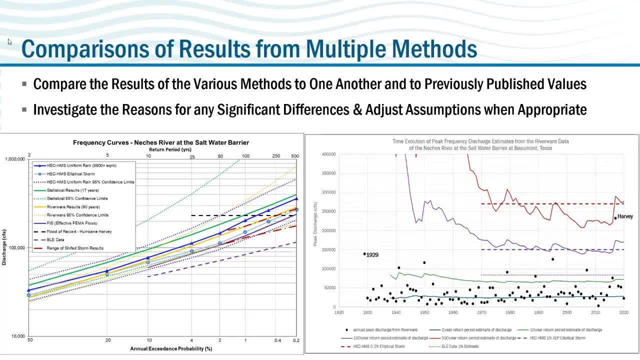 is your traditional frequency curve plot, where you have discharge on the y-axis and probability on the x-axis once again, And we'll have lines from all these different types of analyses that we've ran and compare the results one another, along with some confidence bounds for 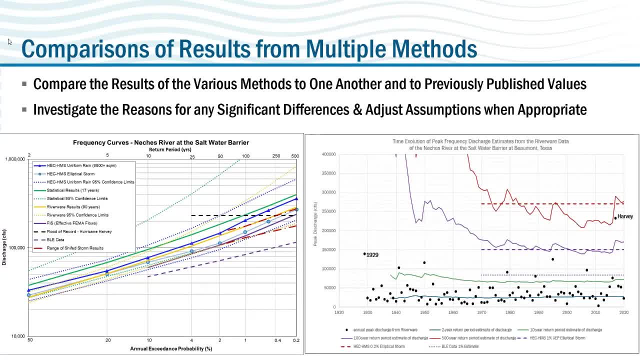 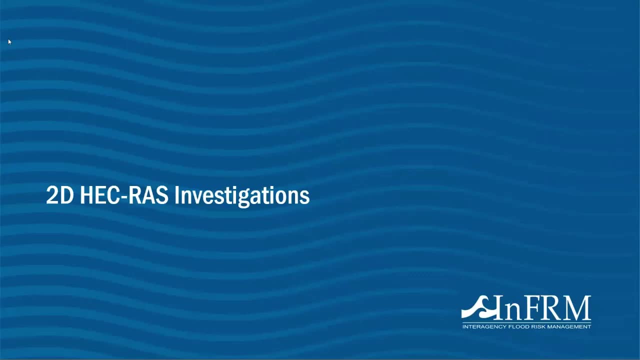 those analyses. We'll also take one of those change over time plots and then plot the model results on top of that and see how that, how does the model results compare to the gauge record, and is it high, low or in the middle? So a 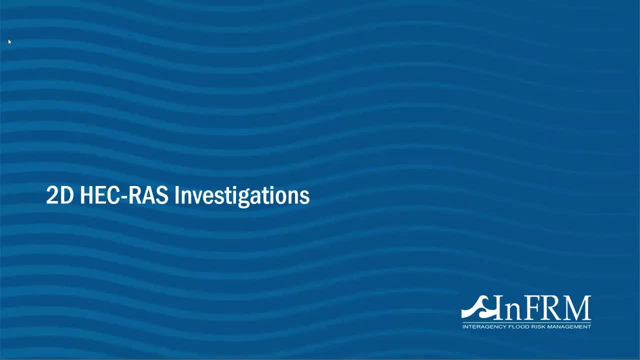 couple of examples I'd like to share with you here. One of the things that we're going to do is we're going to do a lot of emarking and compare checkpoints, And that's a very important parameterə to give you that sense of purity and Jeong-Lan-Wang. 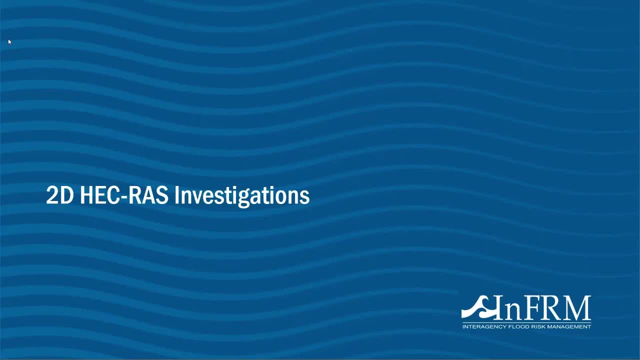 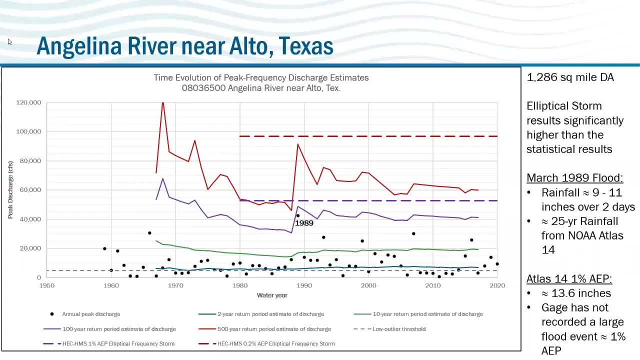 reading relationship and perhaps it will give you an idea of how we're geneitying the trials. So the more analysis, the better our trabajando around people and so taking some narrative surveys and onboarding principle a bit, A couple of experiments that we're looking at: areIG's Timothy. 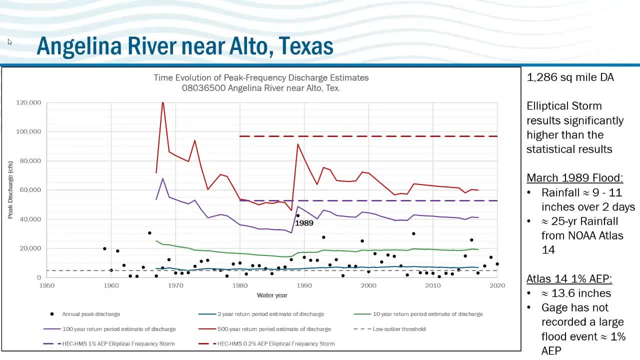 river basin above Sam Rayburn Dam on the Angelina River, and this is a gauge that has about 1200 square miles of drainage area, and this just happened to be a location where our elliptical storm results came out significantly higher than the statistical results for this gauge. 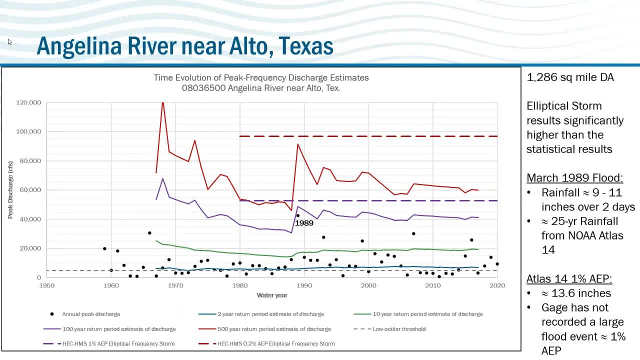 so we started, you know, wondering: well, why is that? well, we started looking a little bit more into the gauge data for this location. we come to find out that the largest flood event that has ever occurred at this location is that 1989 flood. and when we looked into the historic records for that, 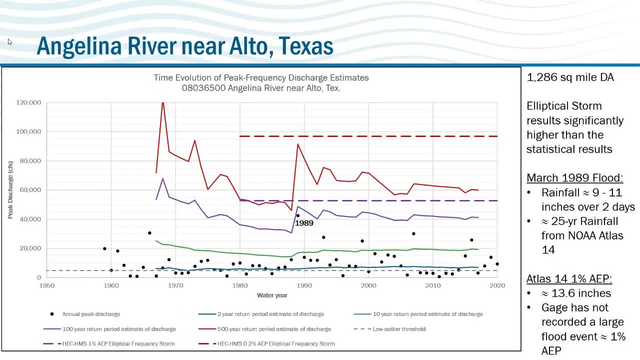 flood, we found that it was produced by about 9 to 11 inches of rainfall over two days, and so if you compare that to NOAA atlas 14, that's about 25 year rainfall event. so that tells us that, even though this gauge has over 60 years of record, it has not experienced anything more intense than a 25-year event. 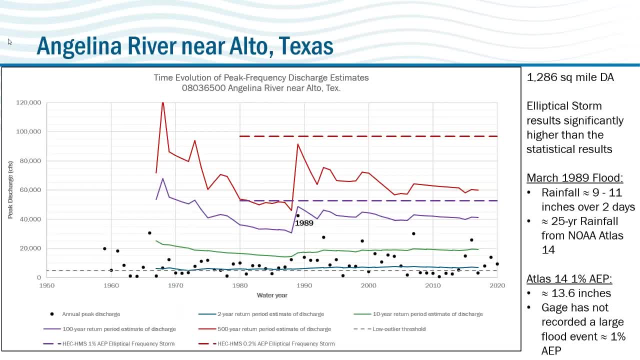 so that's an indication that those statistical results might be skewed a little bit low as a result of that. one of the problems with statistical analysis of gauge records is just that it's very sensitive to sample bias. you have a, you can have a gauge. that's very 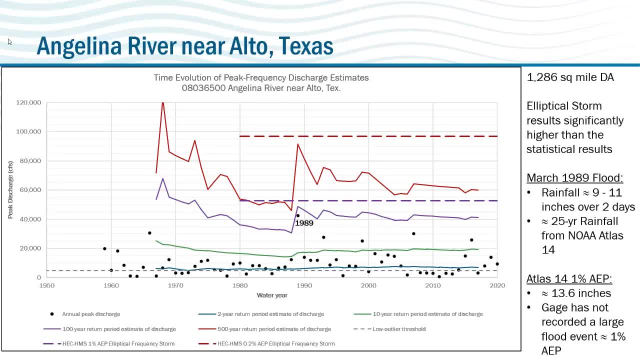 unlucky that has a lot of very large events, you're going to get a very high estimate. you can have another gauge that's been very lucky and has not experienced anything very deep or very intense in terms of rainfall, so that will skew the results to have a lower 100-year estimate. 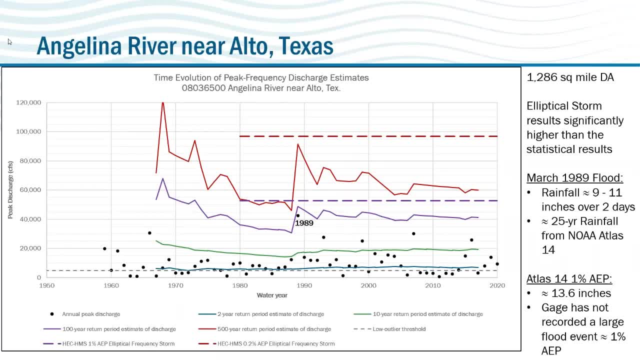 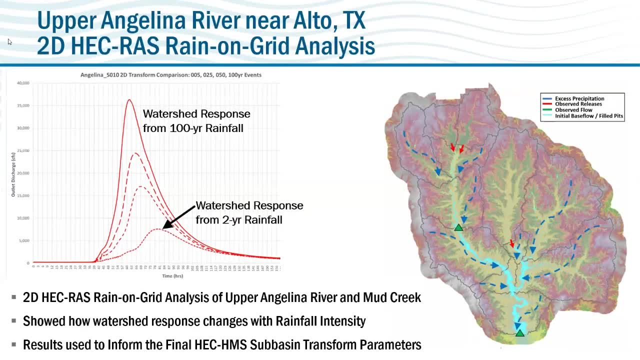 so what we want to confirm once again, you know which line of evidence to believe. more so as a And as a result of that, we also did a 2D HECREV analysis, which is the hydraulic model from the Hydrologic Engineering Center, and basically applied a rain-on-grid analysis. 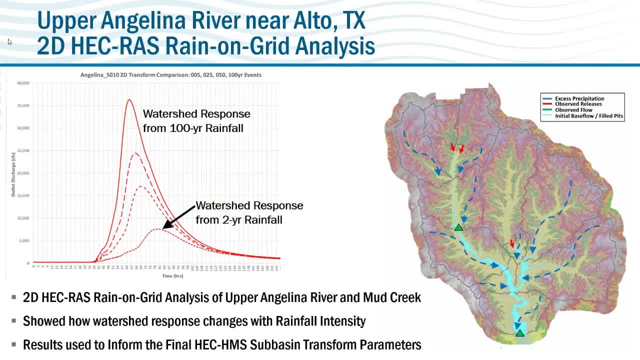 using the LiDAR data for the basin. So the nice thing about the 2D rain-on-grid analysis is you get to account for more completely the physics of how that water runs off, based on a given storm event, And so what this showed us is it helped us capture that difference in the watershed response. 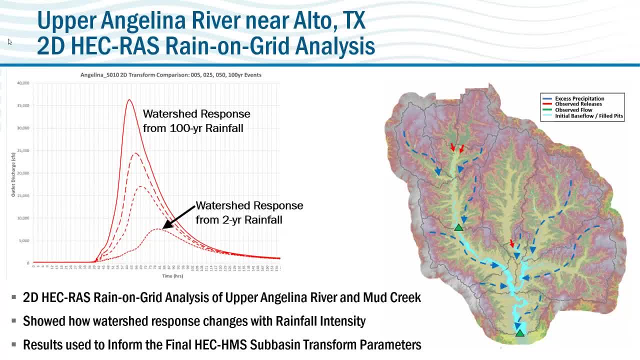 based on: are you getting a moderate rain versus a very intense rain? And so there you see in that graph the difference in that watershed response from a two-year rainfall versus a hundred-year rainfall. The more intense the rainfall, the watershed, the runoff of rain, the more intense the rainfall. 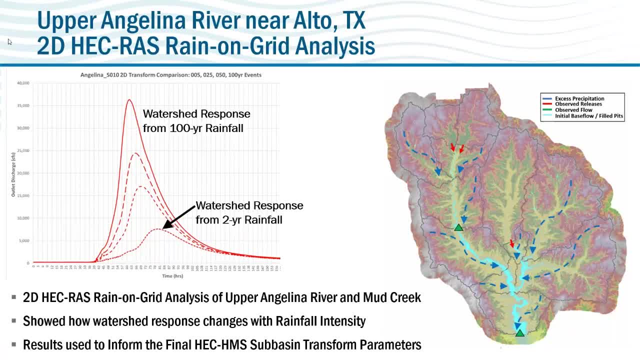 starts moving more quickly, the runoff response becomes faster and more intense, and so we need to account for that when we're trying to estimate a hundred-year flood based on these models. So we used the results from this 2D analysis to help inform the final parameters that were: 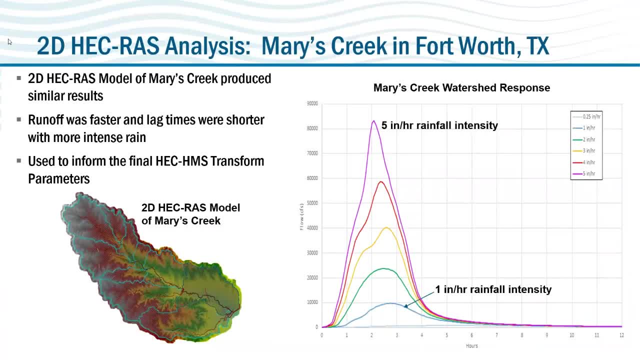 selected in the rainfall runoff model. And then this is another example from here in this area. this is Mary's Creek in Fort Texas, And once again we used 2D HEC-RAS model to help us understand how Mary's Creek would. 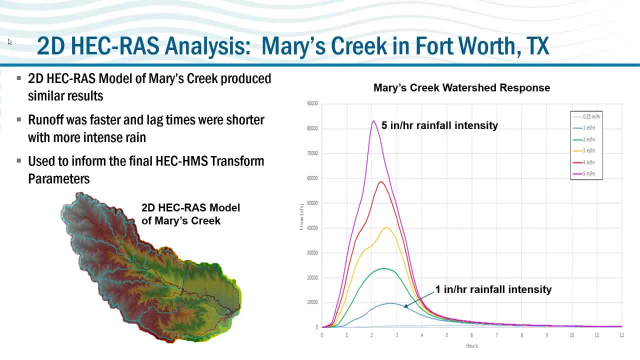 respond for a one-inch-per-hour rainfall versus a five-inch-per-hour rainfall, And this is another watershed that we'll come back to in just a minute- that has not seen a very intense rainfall event from the records that we have available. So finally, another example. 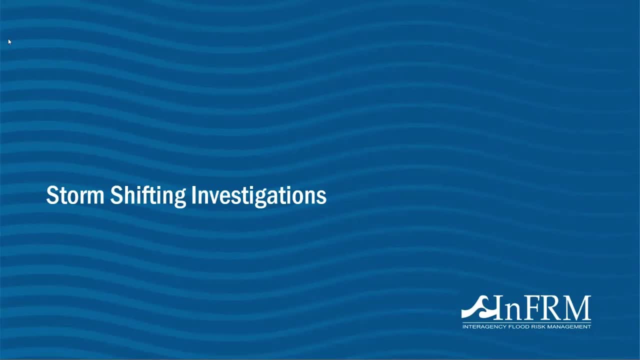 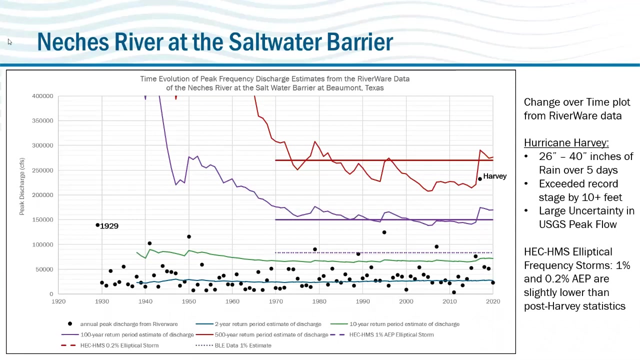 So this is Mary's Creek. Another tool that we have in our toolbox that Jerry talked a little bit about in the last talk was the storm shifting investigations, and I'll show how we use these investigations to help us on the watershed assessments. So this is an example, once again, of the Natchez River, the saltwater barrier, which 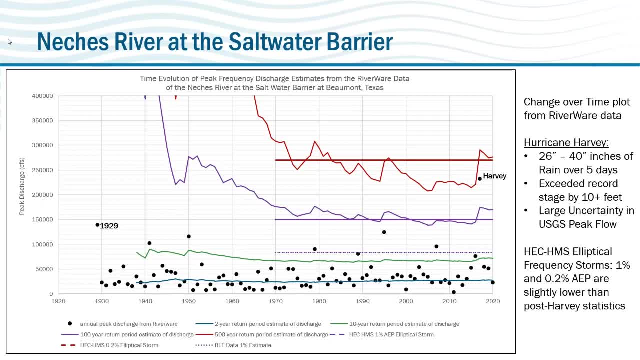 is near Beaumont, Texas. So this is once again one of those change over time plots based on the RiverWare data. and then we overlaid our model. So this is Mary's Creek And of course that's exactly where the storm has landed. 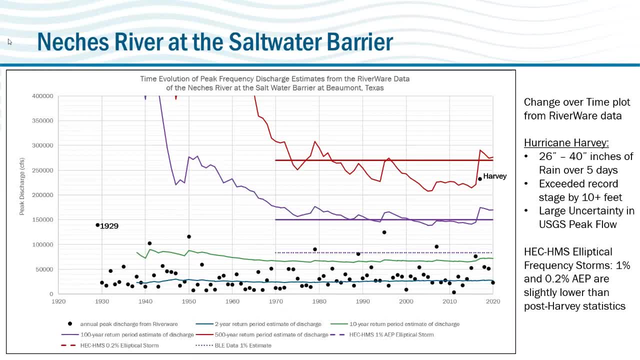 So the storm is in the US. over the last three years, It's all of the Natchez River, and what this means is that the Natchez River has moved over and the Natchez River has moved down. It's generally has moved down 50 or 50 feet, and that's probably where the storm impact. 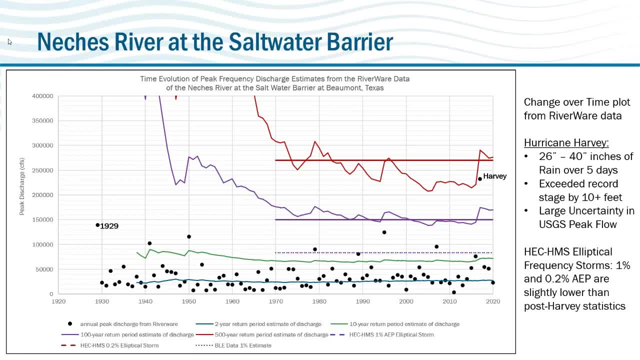 has been, And so the ones here in the Natchez River are the ones that are up here. So my first example is this: this is a storm in the Western Jackson Valley. This is from the final slide, And this is the one we just showed you. And again, there's a lot of thought about this, but we're talking about the Natchez River, in Mauntooth and West Virginia specifically, And this one. here on the Natchez River, you have a storm from the west of Montana and 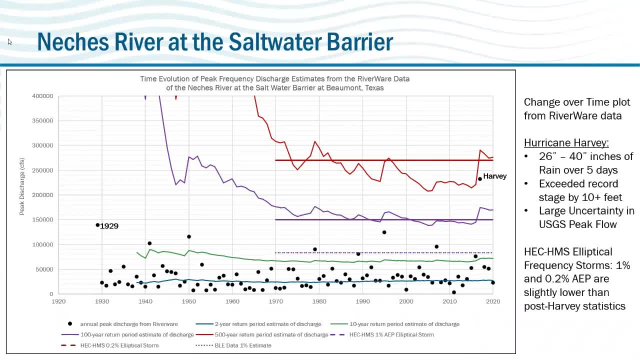 nature's river in this area saw between 26 over 40 inches of rain over five days in that event and um the, the rating curve, the discharge rating curve for this event was exceeded by over 10 feet, so we were trying to forecast during the event and the national weather service, the usgs. 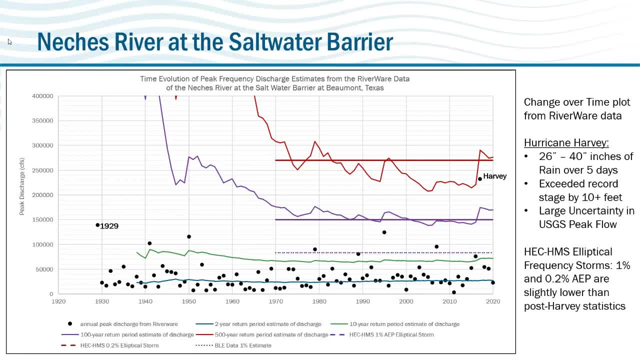 really had no idea what was coming downstream, because it was so far beyond any other event that had occurred at this location. so what we saw here and what, as you can see on the graph, are elliptical storm results from the rainfall runoff model are just a little bit lower than the current. 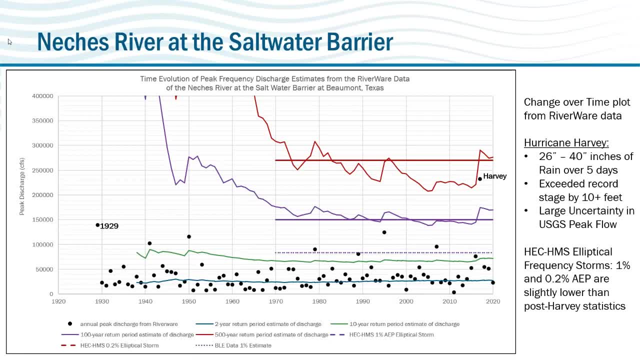 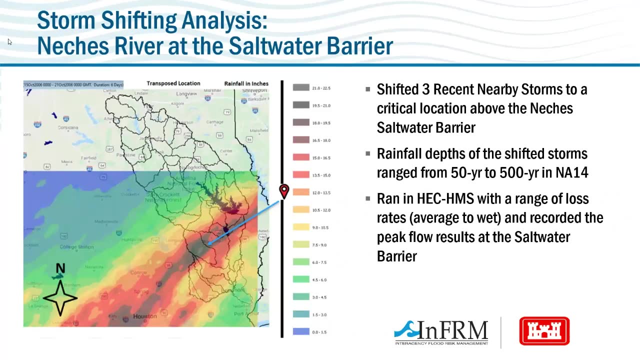 statistical results somewhere we just were looked at that said: okay, which is, which is more true? are the statistics a little high or the model results a little low? so to help us confirm that, we use a storm shifting analysis, so we selected three recent nearby storms that had occurred and 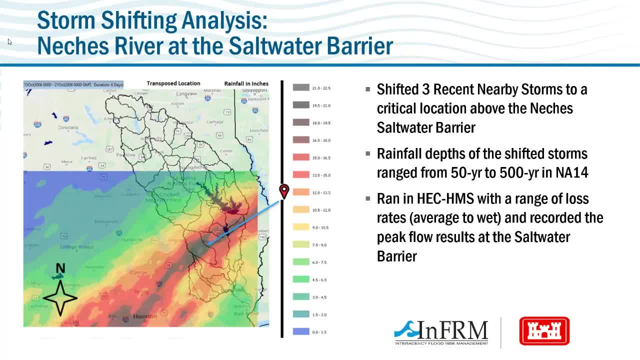 we just shifted them. you know just as the as the hourly records were and the spatial distribution and all that. we just shifted it to a critical location above the salt water barrier. and when i say shifting, we generally just shift, maybe within 50 miles or so. um, from what the position? 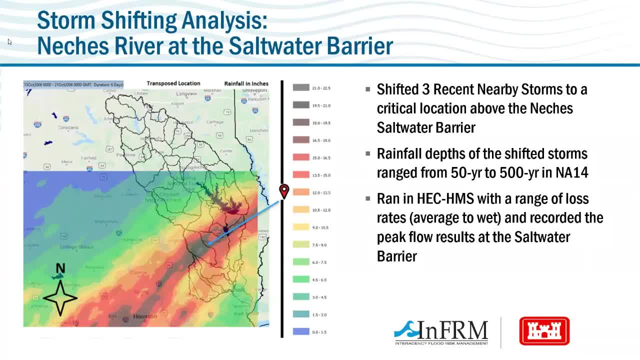 where it's occurred. so the rainfall depth of the shifted storm was a lot higher than the actual rainfall over the last 80 years. we ran้at first year and we ran the shifted storms of the saltwater barrier with a range of soil loss rates. so 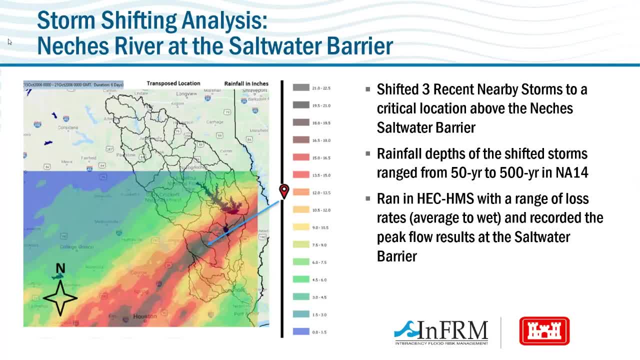 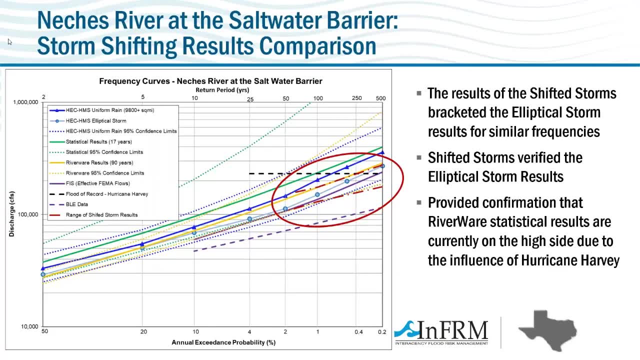 from ranging from average conditions to wet conditions and then recorded the the model results of the saltwater barrier. so what this did is that helped bracket the elliptical storm results from the rainfall runoff model for several months, similar frequencies. So if you look at that graph, the light blue dots are the elliptical. 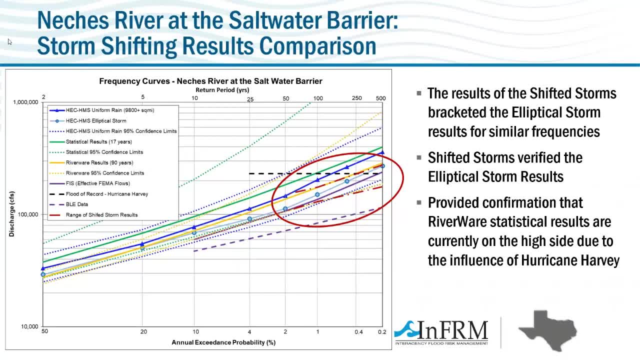 storm results. and then the two red lines that are kind of dotted are the results from those shifted storms. So depending on if you assume average soil conditions to wet soil conditions, it kind of brackets right in the middle those elliptical storm results. So 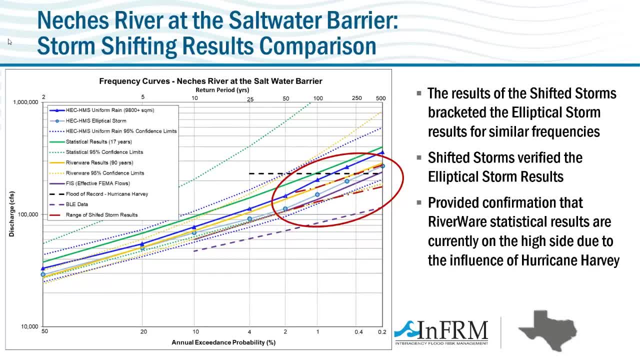 and both of these. it also plotted. the yellow curve on that graph is the riverware statistics. So what this showed us is the riverware statistics are on the high side right now. They're on the very wettest assumptions compared to the NOAA Atlas 14 and the shifted storm results. 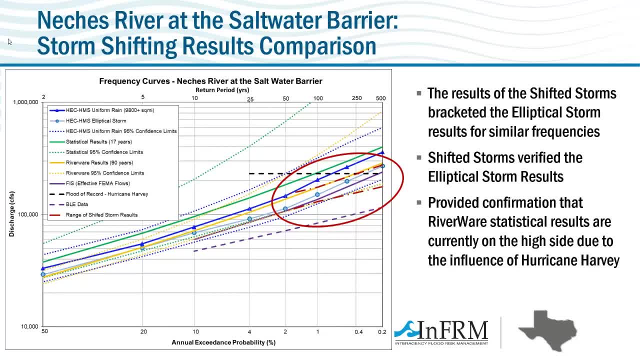 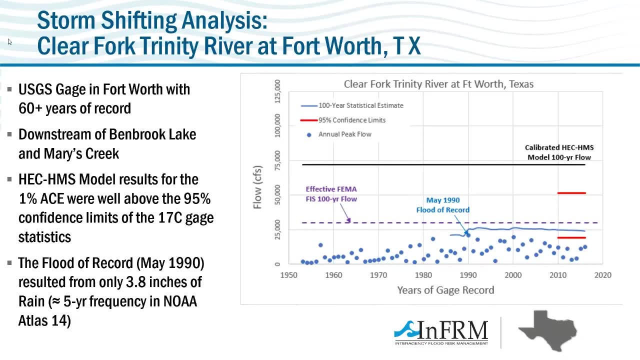 And that's likely due to the influence of Hurricane Harvey. Anytime you have a huge event like Hurricane Harvey in your gauge record, it's going to tend to skew the data and your gauge analysis results to the high side. This is another example. This is in Fort Worth. once again, It's the Clear Fork, Trinity River. 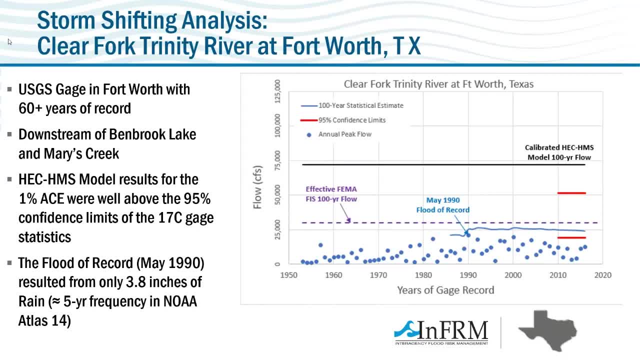 at Fort Worth, And this is another example where we use storm shifting. So this location is actually just a short distance downstream from that Mary's Creek watershed that we spoke about a minute earlier. It's also downstream of Benbrook Lake, which is a Corps of Engineers. 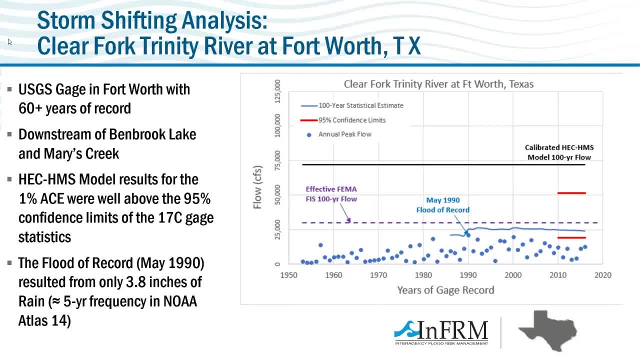 dam That controls a large portion of the watershed. So this USGS gauge has about 60 some years of record. But what we found here was that when we first compared the results, not only was the rainfall runoff model results well above the statistical, it was actually above. 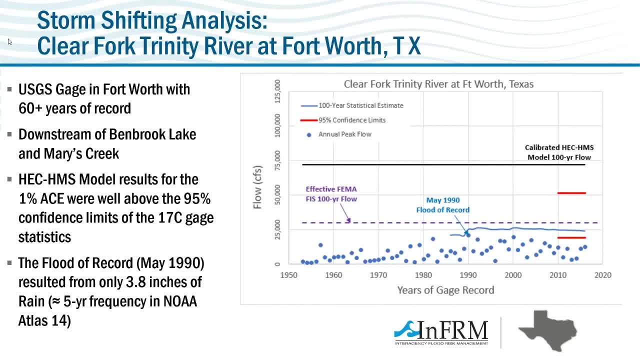 the 95% confidence band of the statistical results. So that caught our attention really fast And that's what you see there on the graph. The blue dots once again are the largest flow that has happened in that year at the gauge And then the blue solid line is the 100-year estimate based on that record up. 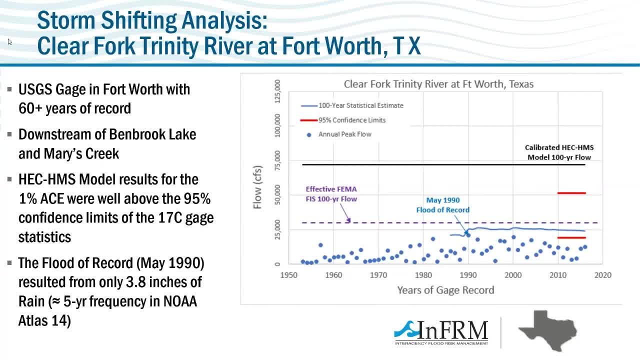 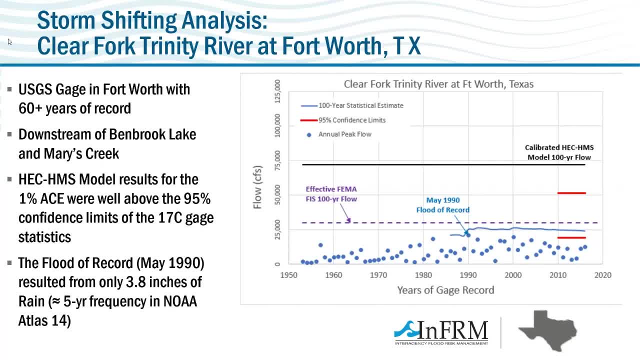 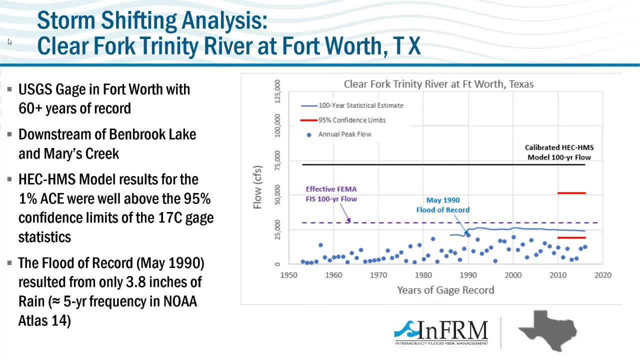 back at the rainfall records only resulted from about 3.8 inches of rain, which is not a very large rain event at all in the Grand Sama thing. So that's about a five-year rainfall according to NOAA Atlas 14.. So this would appear to be a gauge once again that has 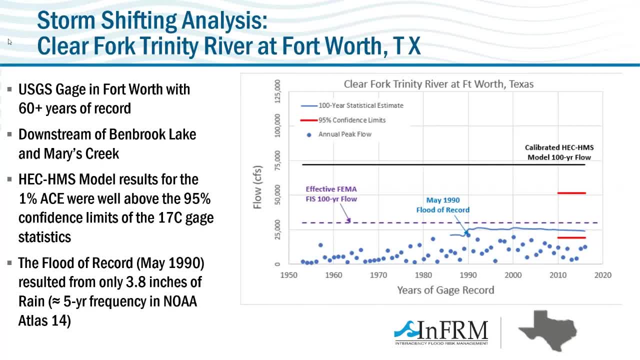 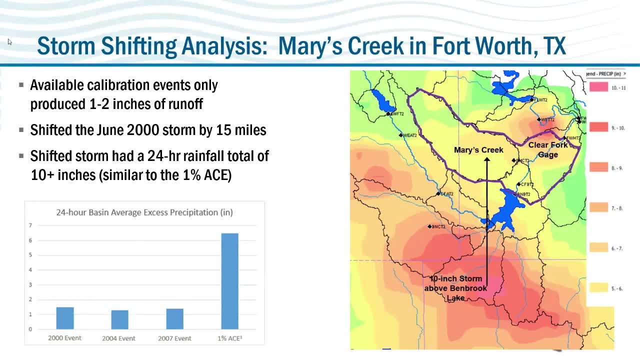 been very lucky So that has just never had that large 10-inch rain that we normally design for. So we did the same type of storm shifting analysis for this also, And so the map on the right is showing to the right-hand side. you see the Clear Fork Gauge, its location. 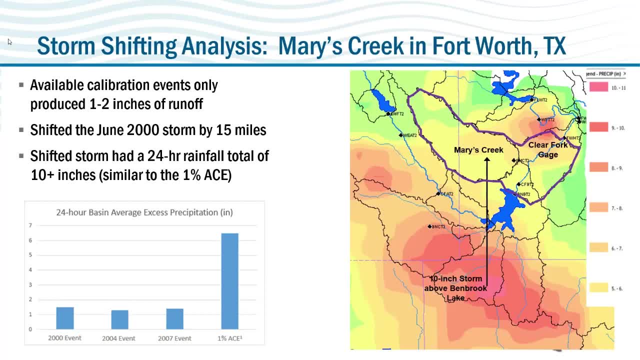 relative to the uncontrolled watershed that is above it, And so Mary's Creek makes up a major portion of that watershed, And then the rest above Benbrook Lake is controlled by the reservoir. So when we looked at this- just that uncontrolled drainage area, we found that the available 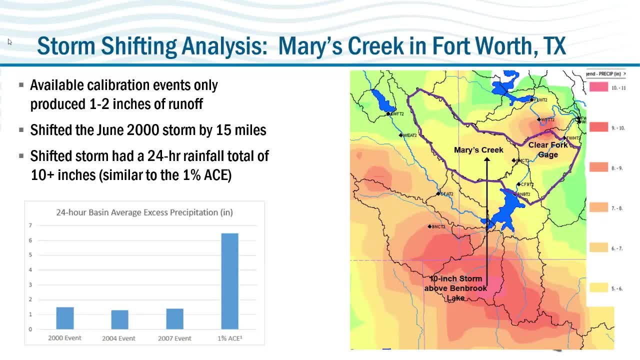 calibration events that we had only produced about one to two inches of runoff, So normally we consider those to be relatively small events. So what we did for this analysis is we actually took a June 2000 storm which had a 10 inches of rainfall that fell above Benbrook Lake, And then we took a June 2000 storm which 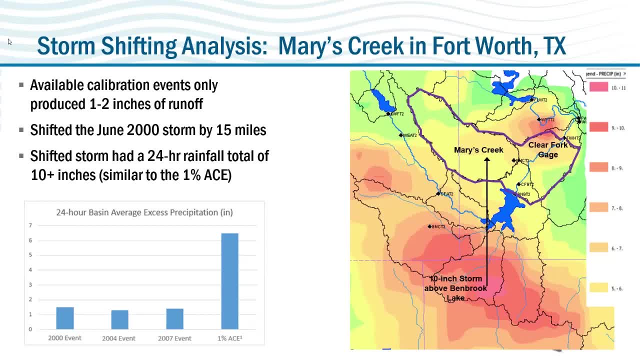 had a 10 inches of rainfall that fell above Benbrook Lake. And then we took a June 2000 storm, which had a 10 inches of rainfall that fell above Benbrook Lake. And then we took a June 2000 storm which had a 10 inches of rainfall that fell below. 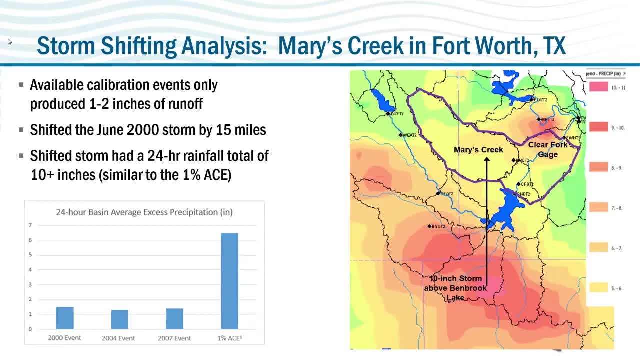 Benbrook Lake And then we took a June 2000 storm which had only enough rainfall And then during the actual event, that rain was just absorbed into Lake Benbrook and it never. it was released very slowly So you never saw a large flow to the Clear Fork Gauge. 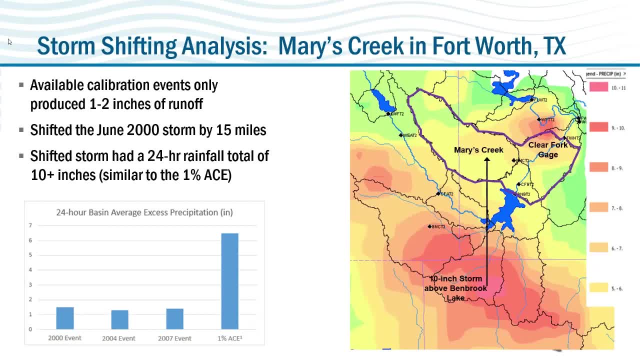 So we just did that event and we just moved it 10 miles north or 15 miles north to Mary's Creek as the what if? What would have happened if that 10 inch rain happened 15 miles north instead of where it did? 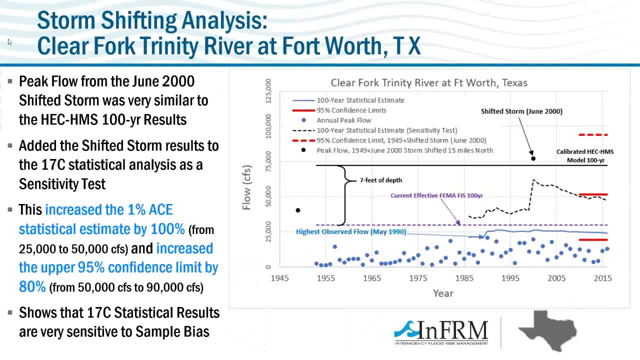 And what we found from this is that the model results that we found at EAC are very similar from that June 2000 shifted storm were very similar to the rainfall runoff results from the 100-year storm that we had run earlier, and you'll see that on the graph on the right there. 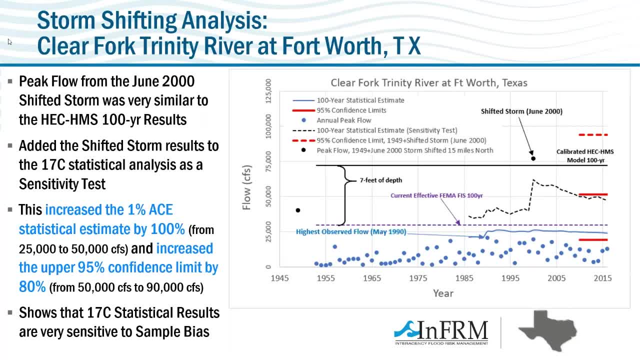 you see that black dot is the June 2000 storm on the right which is just above the calibrated HMS model results for the 100-year. we also, as a sensitivity test to the gauge analysis, the 17c gauge analysis, we added that shifted storm back into the bulletin 17c statistical analysis. 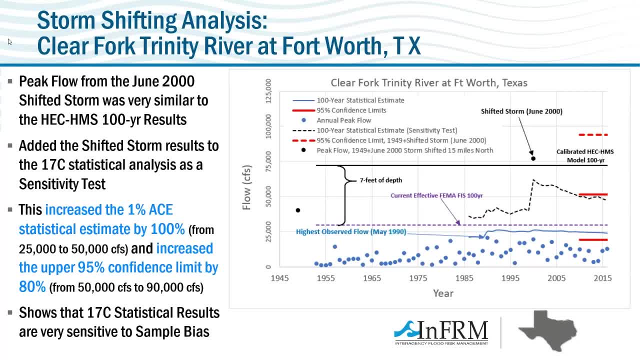 just to see what would happen. and just adding those shifted storms increased the 100-year statistical estimate by a hundred percent. it doubled from 25,000 CFS to 50,000 CFS. and even that 95 percent confidence bound, the upper one moved up by 80 percent, increased from 50 to 90,000 CFS. so this just confirmed just how sensitive. 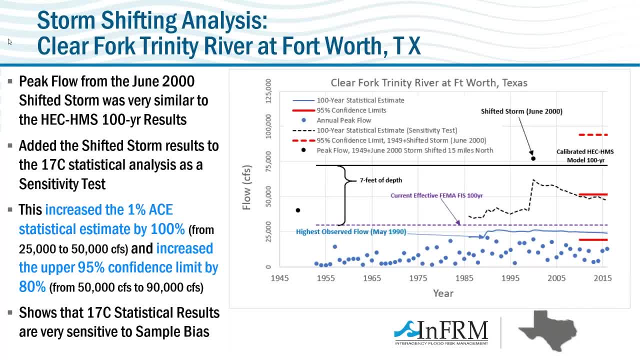 those gauge statistics are to one or two events that they have occurred slightly differently at slightly different locations could have produced very different results at this location. so once again, that 17c statistics are very sensitive to sample bias. it assumes that you've had a representative sample of flood events that occurred in that watershed. 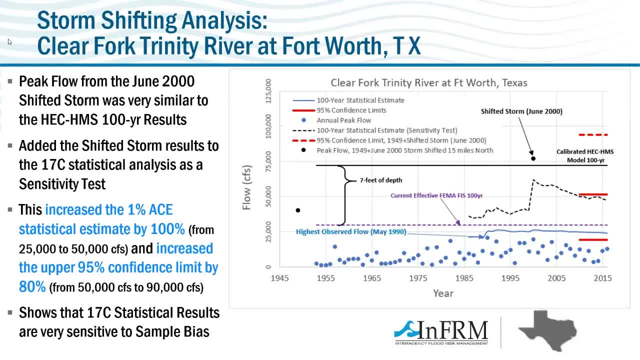 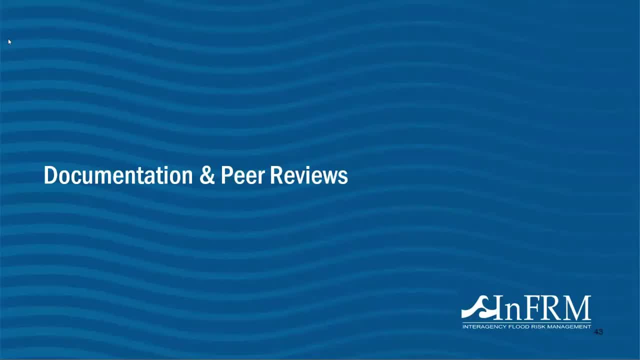 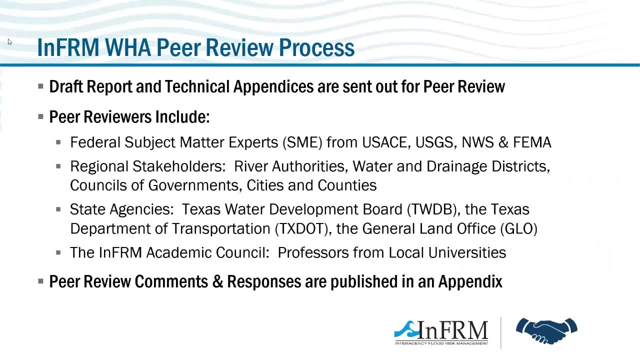 which you could have actually been lucky or unlucky depending on the type of events that happened there. all right, so that's most of the heavy technical stuff after we get through all these different types of analyses. so once again, we try and include water resources and hydrology. so we're we. 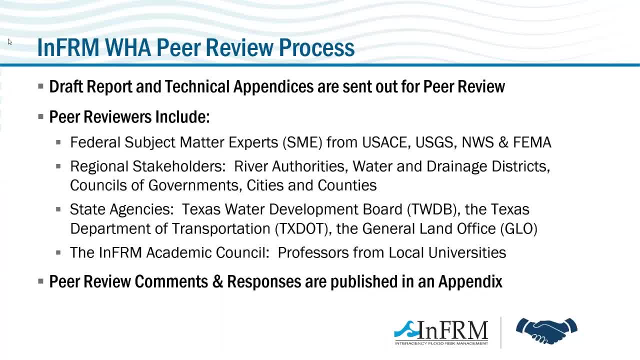 put out draft report and technical appendices, summarize all this and we send it out for peer review, and so we try and include different experts and watering systems on hydrology from across the state to participate in the peer review process. so we'll have subject matter experts from the different federal agencies to 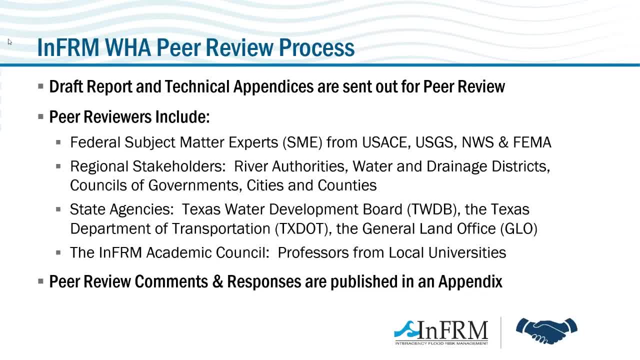 review it. we'll have regional stakeholders, which may include river authorities, water and drainage, and counties, different stakeholders in that basin, as well as different state agencies, including the Water Development Board, TxDOT and the General Land Office. We also participate with what we call the Informed Academic Council, which is just a grouping of professors from different universities. 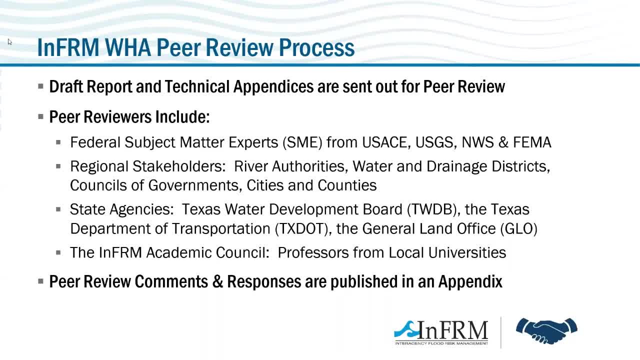 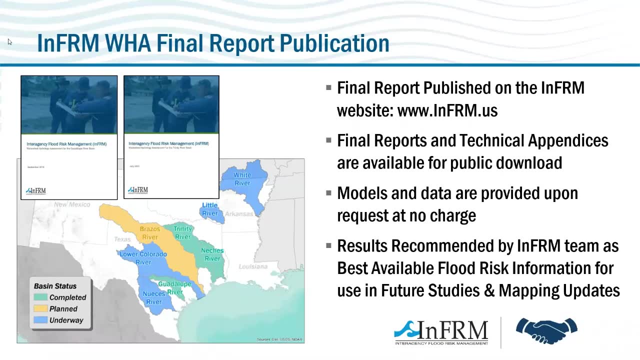 across Texas that participate in this peer review process with us. So the peer review comments that we receive and the responses are published with the report in an appendix, And then the final reports from these studies are published on this Informed website and these reports and appendices. 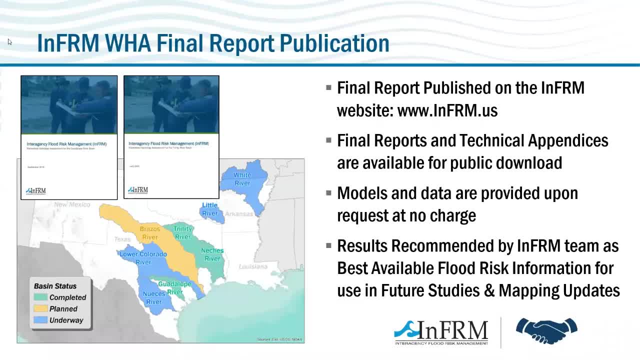 are available for public download. We also make the models themselves available at no charge. They're provided upon request, so you just have to reach out to us, And these results from these studies are recommended by this group of federal agencies as best available flood risk information for use in any future studies. 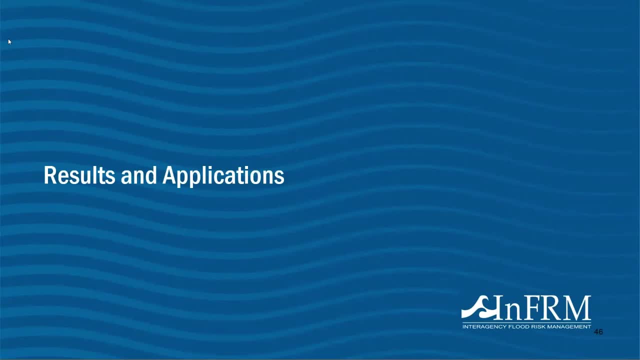 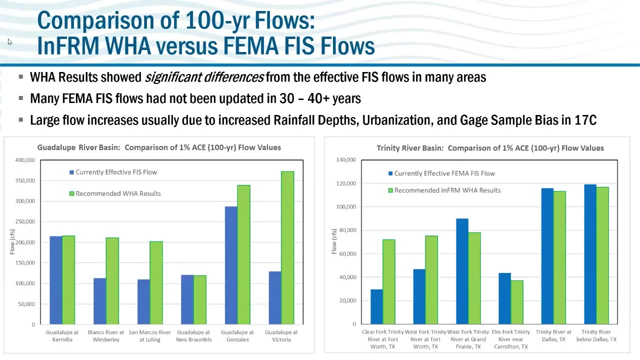 So finally, just some results and applications from these studies. This is just a comparison of the 100-year flow results from the Informed studies versus previously published FEMA flood insurance study flows, And what we saw is that there are significant differences from the Informed studies versus the FEMA flood insurance study flows. And what we saw is that there are significant differences. 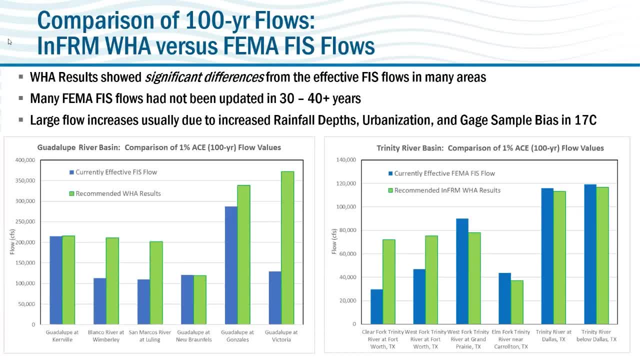 from the effective flood insurance studies in many areas, but those differences vary. they're somewhere much higher, somewhere it's much lower, somewhere it's about right. and that's where these bar graphs are showing just different selected locations, where the green is the inform watershed estimate and then the blue bars are the currently effective. 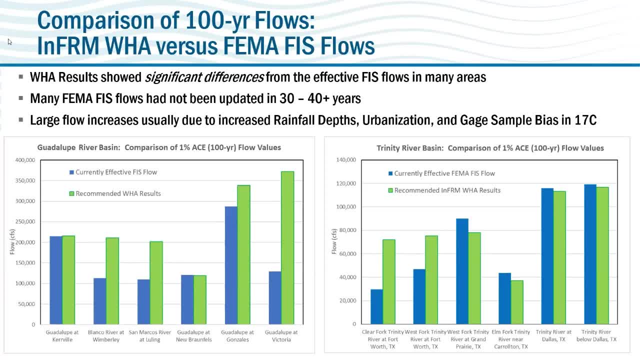 flow, 100-year flow for that location. but one of the things you know that we see over and over again is a lot of times, the flows, the hydrology behind the current FEMA maps for a lot of these large rivers has not been updated in 30 to 40 plus years. so even when FEMA's putting 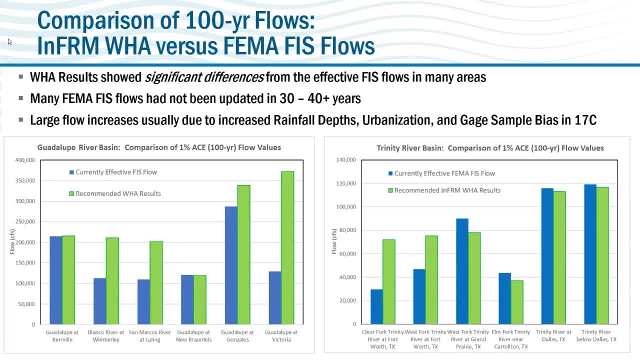 out new mapping updates and modernizing their maps. a lot of times they never go back and update the hydrology. they'll like update the lidar, they'll update a new hydraulic model, but those flows still go back 40 years and are just carried forward in many cases. so some of the reasons that we see for the, the differences, and especially where we 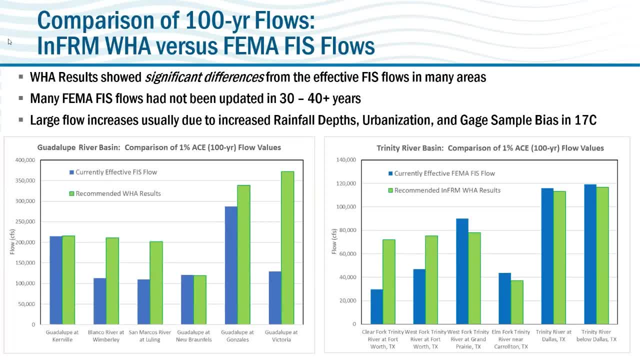 see an increase in the 100-year flow. a lot of times it's due to rainfall depths, as Jerry alluded to those. NOAA Atlas 14 had significant increases down near the Gulf of Mexico as well as in southern Texas and near the hill country. it could be due to urbanization in an area like this especially. 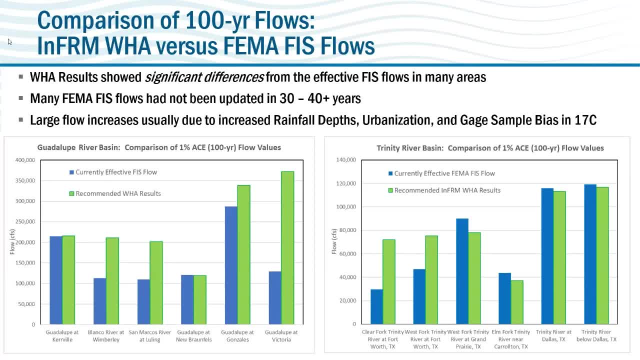 that's undergoing rapid development and then also it can be due to that gauge sample bias from 17c. there's a lot of FEMA studies that are just based on the bulletin 17b or c analysis that were done at that point in time and so if that hasn't been updated in 40 years, 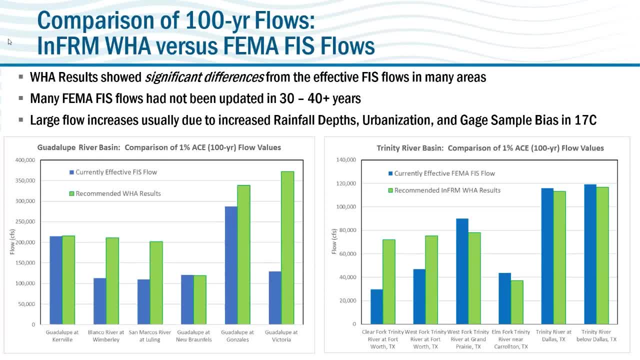 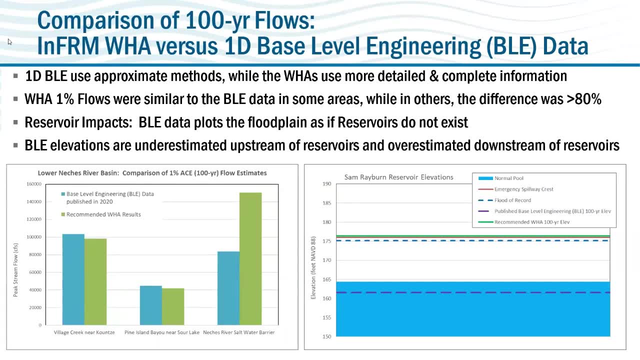 you know you can have a lot that's happened since then that would change that estimate. another comparison we've looked at is to the base level engineering data and that's that. that's those approximate HEC-RAS models, and the HEC-RAS models are available from FEMA and the 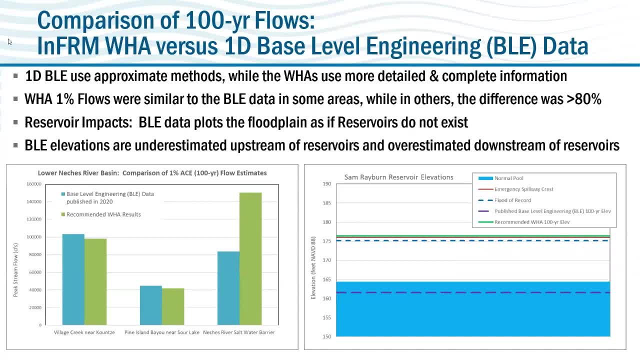 InForm website and those are good models. they just use approximate methods for the hydrology behind them, and so we compare those. there are areas where the flows came out pretty similar and there's a lot others where the difference was over 80 percent, and that's what that bottom left graph is showing. 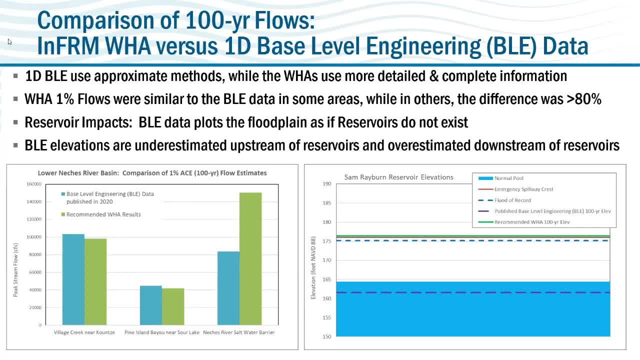 just differences at different locations in the nature basin, but one of the big things to be aware of if you're using that base level engineering data is that it does not account for reservoirs. and so we, we know they say in the in the notes: it doesn't account for structures and it's you know. 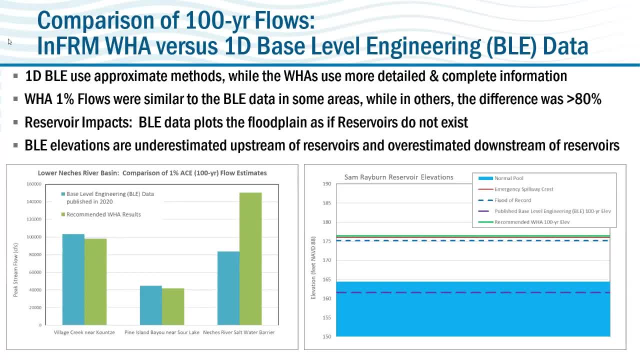 most of the time we think of bridges, culverts, things like that. it's one thing not to account for, another thing not to account for bedbrook lake or lake louisville. so what that data plots is it'll. it'll plot the floodplain as if those reservoirs do not exist. so the that plot on the lower right. 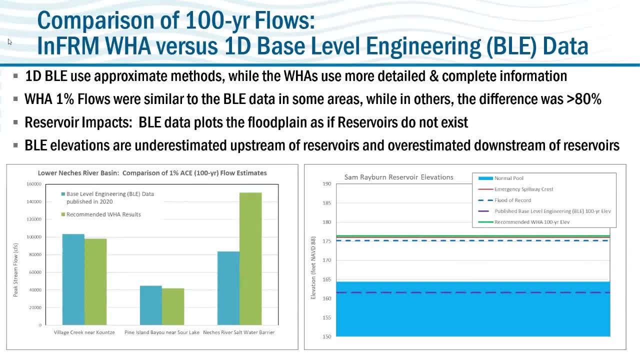 is showing a comparison to the ble data at sam rayburn reservoir, which is a core of engineers reservoir in east texas, and it's actually plotting the 100-year lake elevation at below normal pool for that lake. so it's way low, whereas the analyses that we did had it way up near the flood pool and near the. 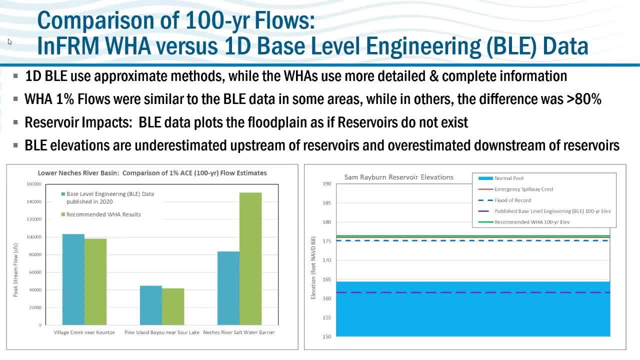 emergency spillway crest. so what this has the effect of is those ble elevations are much too low upstream to the dam and a lot of times they're too high downstream in the dam because they don't account for any of the flood risk management effects of the reservoir downstream. 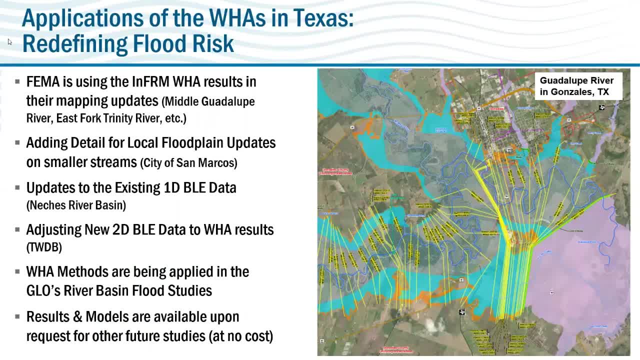 some other applications of how these watershed assessments are being used. in texas, fema is using them to update their hydrology and any of the new mapping updates that they're doing across the region. so some examples. this has already been applied in the mid. for the middle, 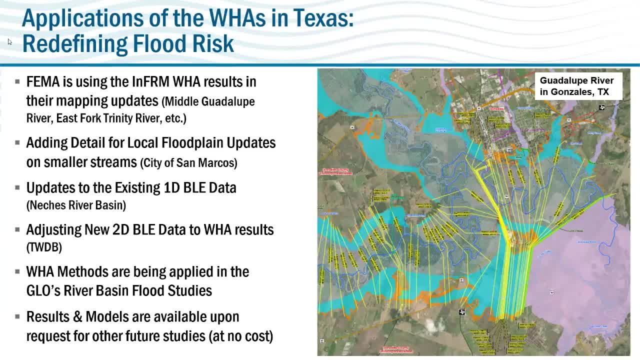 guadalupe river, and that map on the right is showing you the new results that incorporate the inform hydrology into the guadalupe river modeling. that's near gonzalez, texas, and then they've also been implemented in the east fork, trinity river and river near rosser. 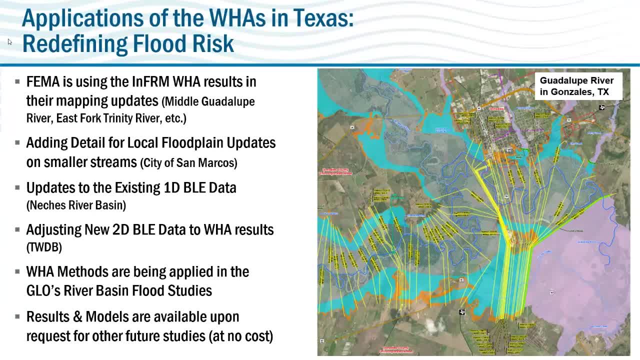 in this area and they continue to add on as fema has budget and planning for different mapping updates. we also use them to help communities add detail for local floodplain updates on smaller streams in some of these basins. so this is a really good example of a lot of the new data that we've been able to get from the city of san. 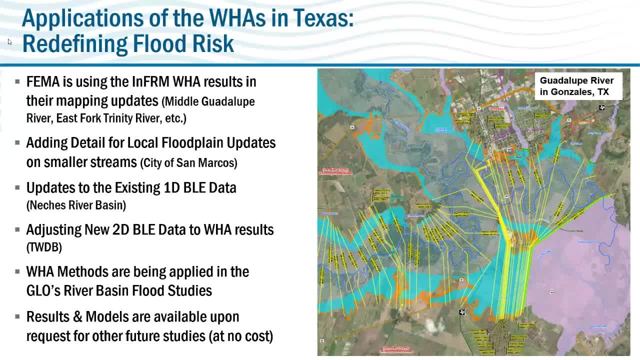 marcos. one example is the city of san marcos. you know we studied the guadalupe river basin but you know, could only go to a certain level of detail, and so the city of san marcos asks us to help just update their floodplain and their hydrology for some of the smaller streams in the 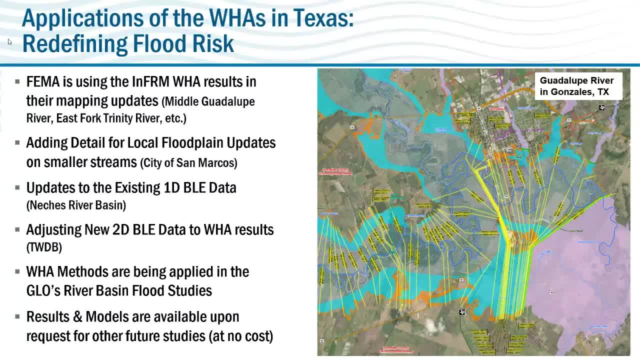 basin so we're able to apply some of the same methods from the hydrology assessments to come up and then we can start to do some of the more detailed water assessment for some of those smaller tributaries. we're also looking at updating some of that ble data to take more detailed. 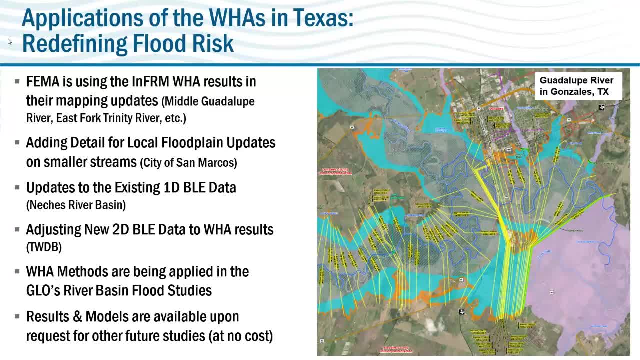 hydrology information and put it into those hydraulic models so we have a better estimate available on on the ble data and we're working with the texas water development board and they're actually taking wherever we have a watershed assessment that's published and where they're taking the data they are um dictating to their contractors. hey, you guys need to check. 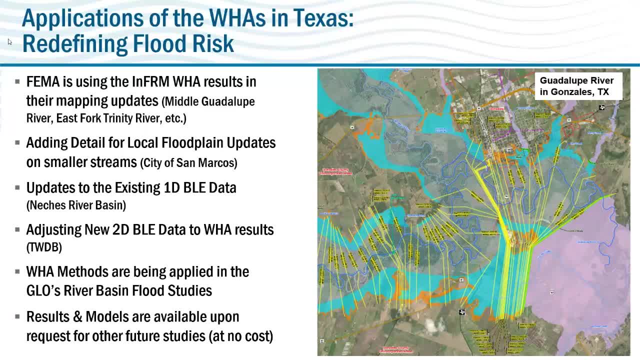 the flows that you're coming up with against these, these other hydrology results, to make sure that they're um with their alignment with one another. these methods that we're talking about today are also being applied in the texas general land offices- river basin flood studies. some of you may have heard of those. they're being done for a large 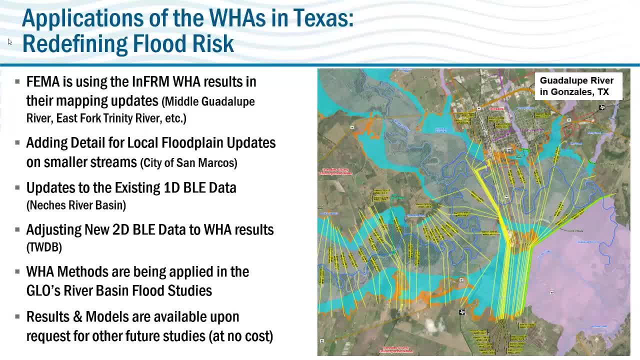 number of years now. we're working with the reas management to make sure that they're available for use and then, as i mentioned, um, we have an estimated 90s or so flood risk management studies, which are all done in south texas, and we're also doing conductive monitoring. 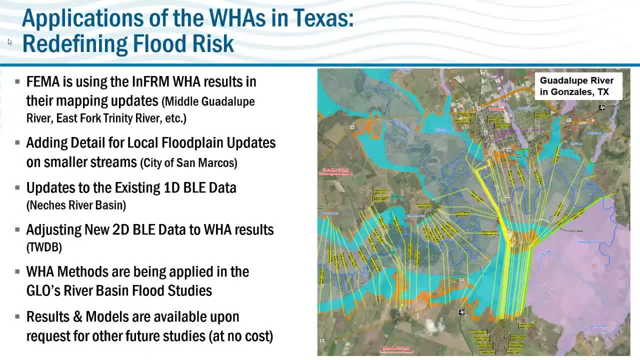 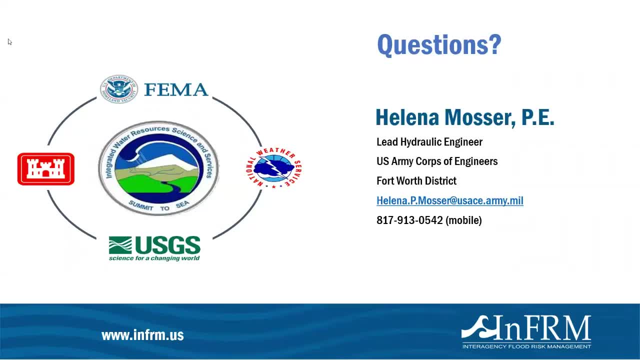 there's kind of a general kind of spot of texas, especially along the coast, where they're doing a lot of planning and um flood risk management studies in those areas, and those studies are using a lot of the same methods that we've talked about today. if you'd like to follow up afterwards with any additional questions, 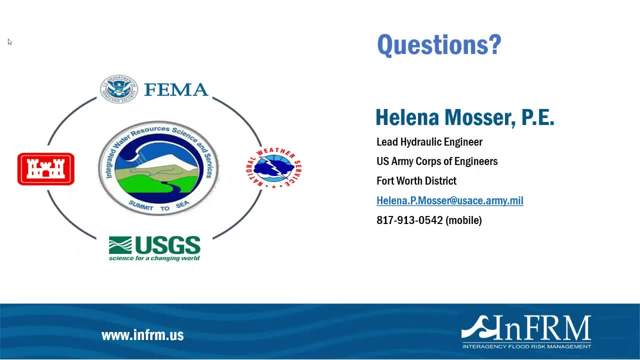 Yes, How often do you think those watershed hydrolithics will be updated? and I know you said the new TLE data might incorporate them. Do you think they would go back and update, since those are the TLEs? There is a plan to do that As far as when to update the overall watershed? 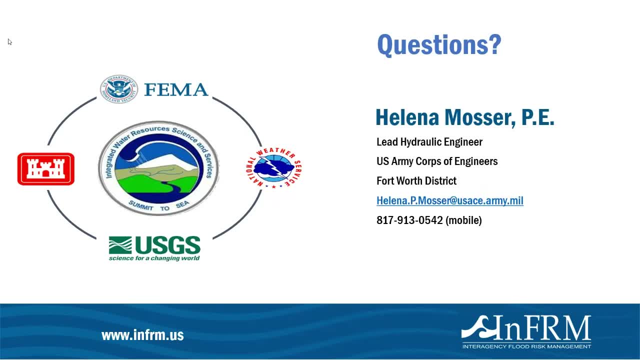 hydrology assessments. I think it's going to depend, It's going to vary by basin, because not every basin is experiencing as rapid development as, say, Dallas-Fort Worth is. But we are also looking at incorporating, as an addendum to these studies, another estimate of future hydrology. So 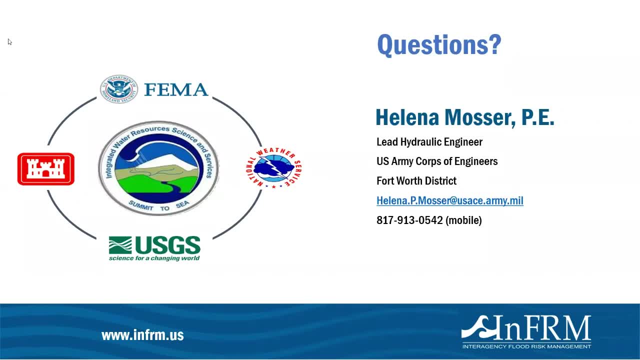 looking at future land use so we can have at least an existing and future estimate for future development. Yeah, and then the BLE data. That goes in cycles depending on the who's funding it. So so far it's been FEMA and the Texas Water Development Board that have funded those studies, So they're on like a five to ten year cycle, Right? 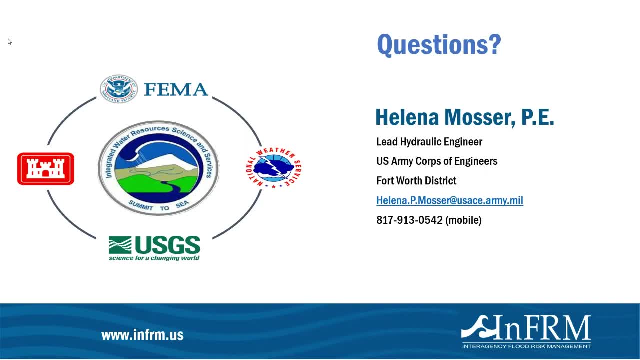 now they're just trying to get all of Texas modeled and, you know, get something out. But once they get, you know, the whole state covered, then they'll go back to the beginning and say, okay, what needs to be updated, and start bringing in some of those updates, those models. But I would say 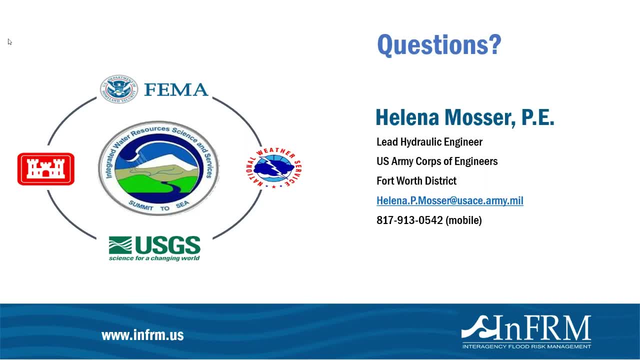 probably a five to ten year cycle. So usually it depends on the funding source or the customer right. So these studies that we're doing for FEMA, FEMA doesn't necessarily look at future ultimate conditions, But if we're partnering with a city or county- somebody that does- then yeah, it's fairly simple to take. There's only as many parameters. 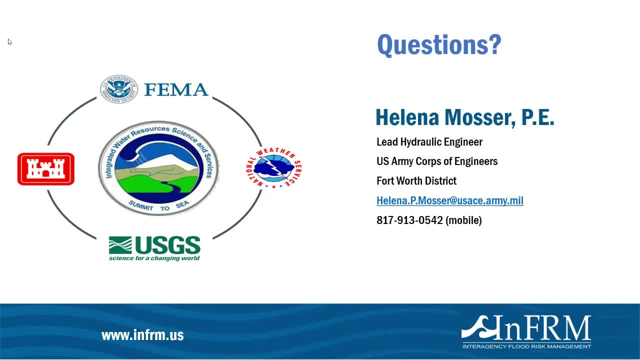 that have to be updated, to take out that modeling and then update it for ultimate conditions. Right now for the Trinity we're working with the North Central Texas Council of Governments And so they have an estimate of land use for like 2055.. And we'll use that. It's not ultimate but it's at. 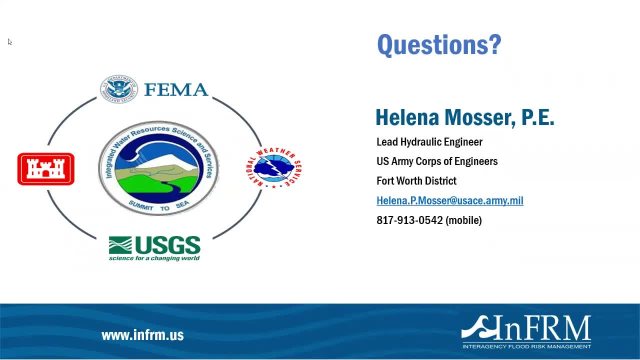 least a point in the future that we can reference, that this is the existing flows and this is what 2055 might look like. So that's what we're working on right now. So that's what we're working on right now. So this is the existing flows and this is what 2055 might look like. 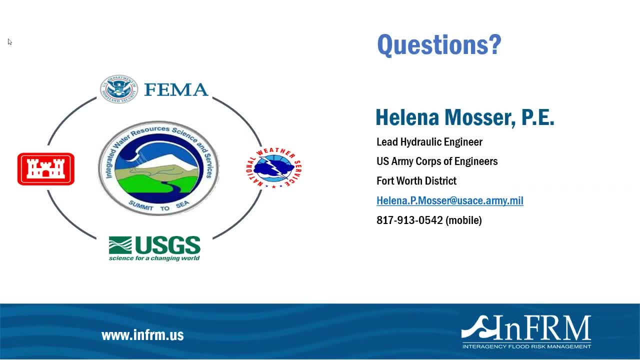 Yes, Is that 2002?? Uh, Or a 90?, 98? Okay, yeah, October 98 on the Guadalupe River was a huge event, So it kind of depends on where, exactly what. what point you're looking at on the Guadalupe River. 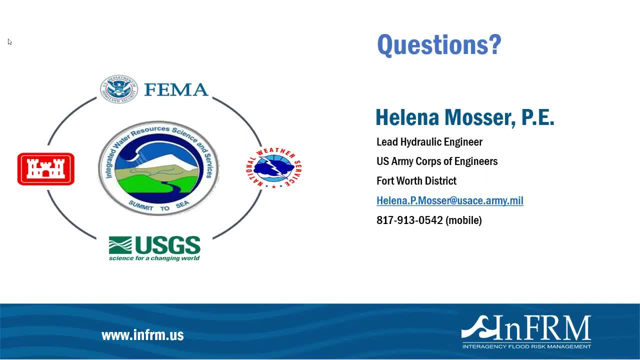 Yeah, so I think those were at least a hundred year event, Maybe more. And then by the time you got down further downstream to like Victoria, it's more like a 200 to a 500 year event. Because it got down further downstream to like Victoria, it's more like a 200 to a 500 year event Because it got 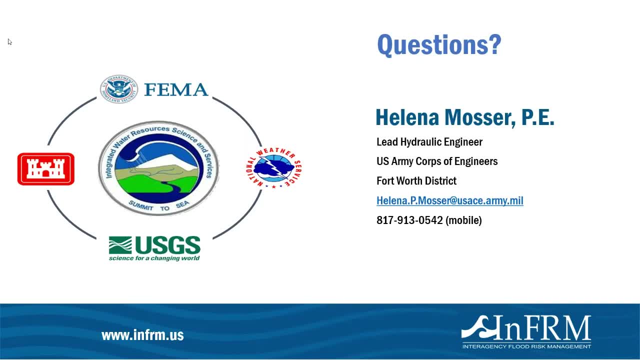 anywhere between 20 to 35 inches of rain in that October 98 storm event at different locations in that area. So it was. it was a monster storm event: anywhere between 20 to 35 inches of rain in that October 98 storm event at different locations in that area. So it was. it was a monster storm event. 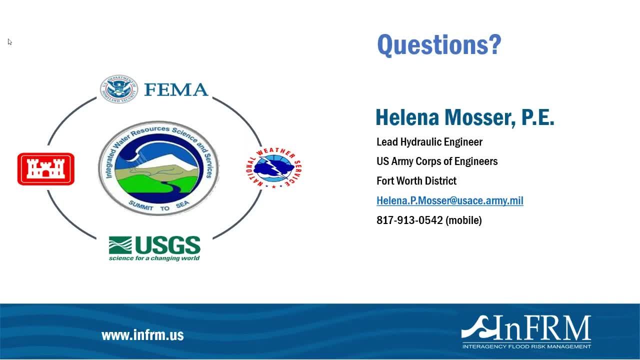 Was that the? was that just because of it just deployed, or like a Right? yeah, we used that storm as one of our calibration events, so we we used that to try and make sure our model was matching what happened in that storm event. Right, yeah, it's, it's incredible. 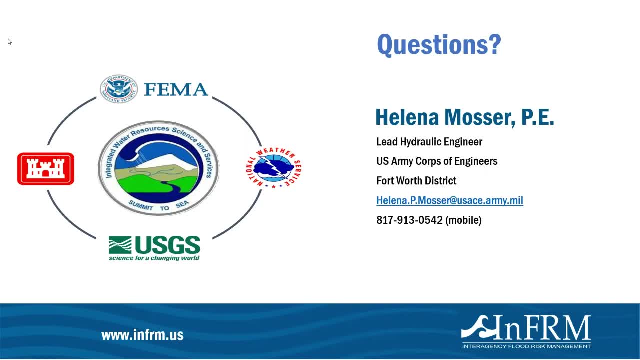 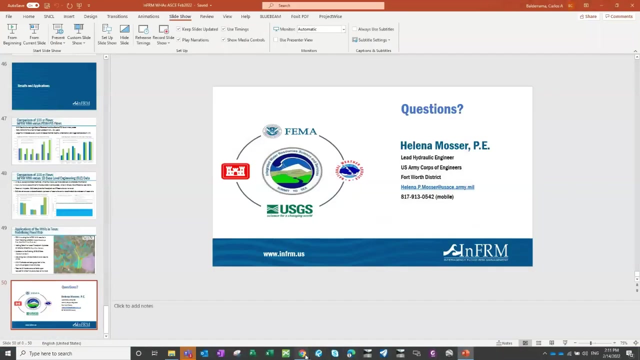 Any other questions? All right. thank you Awesome, you did awesome.